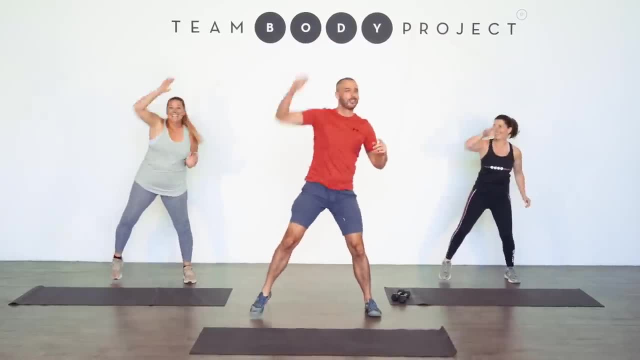 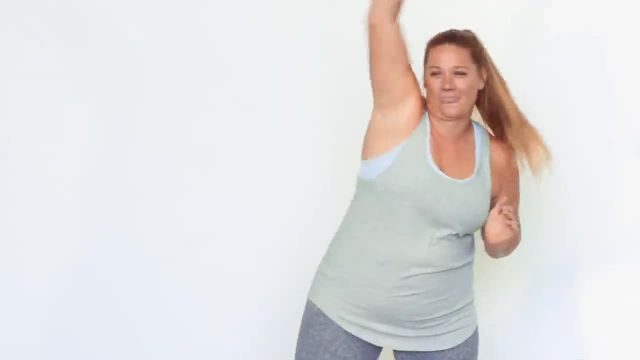 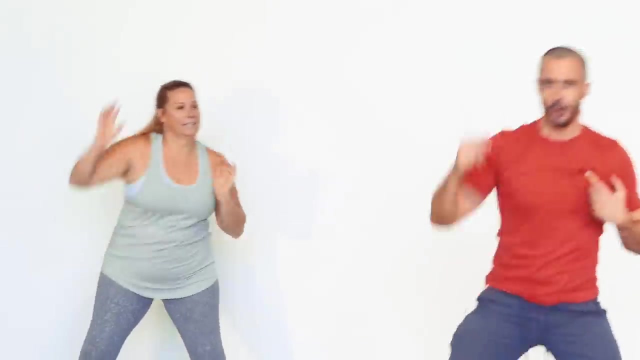 Well, maybe you're just questioning what you're doing. stood behind this strange chap who probably talks too much Dip and reach Nice and high, And I think that that's the central focus of this whole plan is: I want you, we want you. 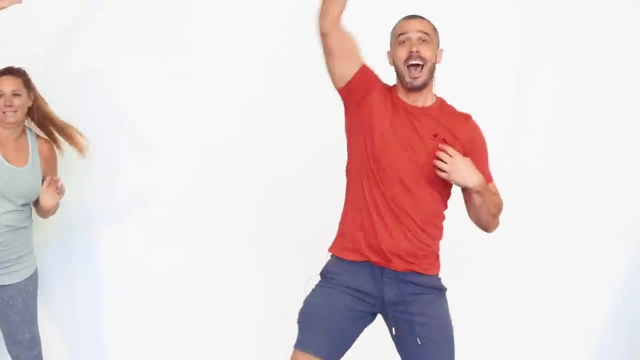 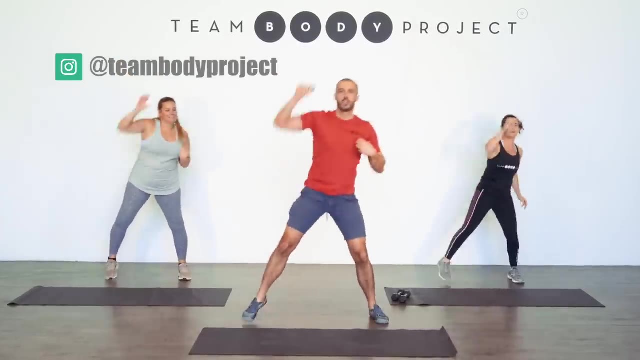 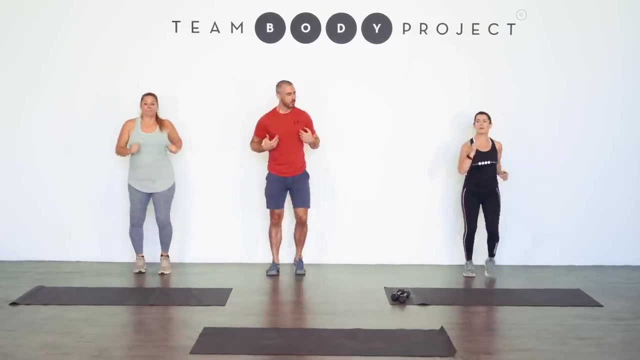 to work out with us at your pace and really enjoy taking part in the session Three, two, one And a little march and a nice deep breath And a nice deep breath. So everything runs at 30 seconds with an active recovery. 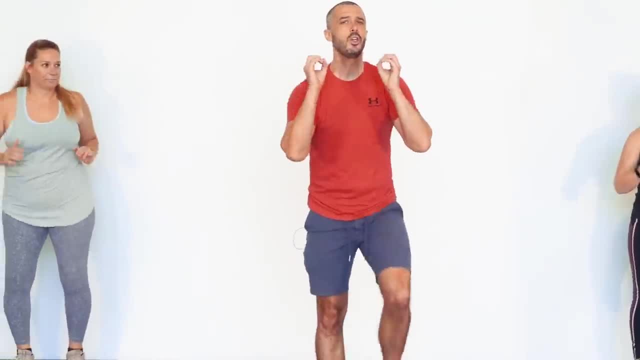 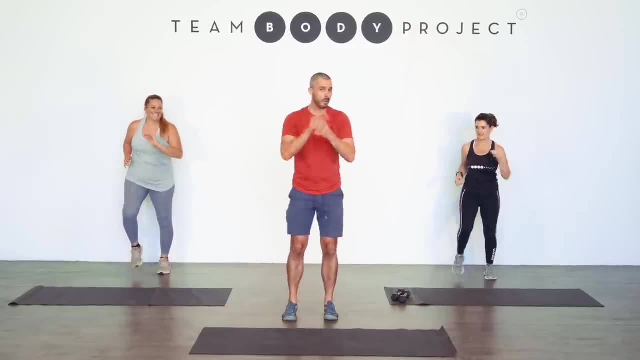 And in the active recovery you're going to give what you choose to. Does that make some sense? I'm going to guide you. We're going to start with the first exercise of 30 seconds and it's going to be a side lift with an upper cut. 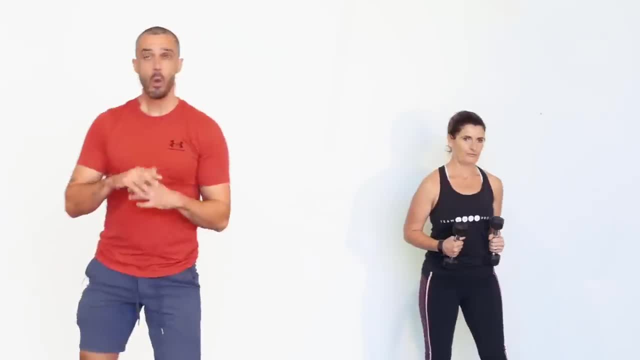 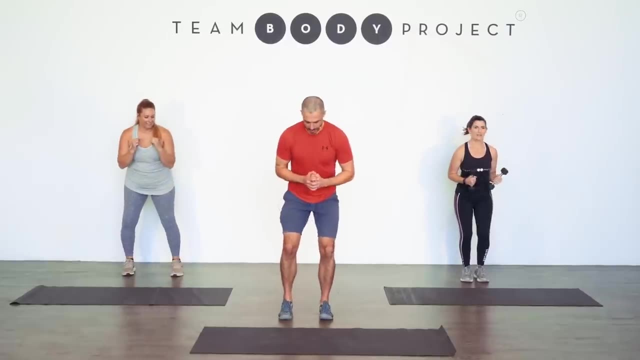 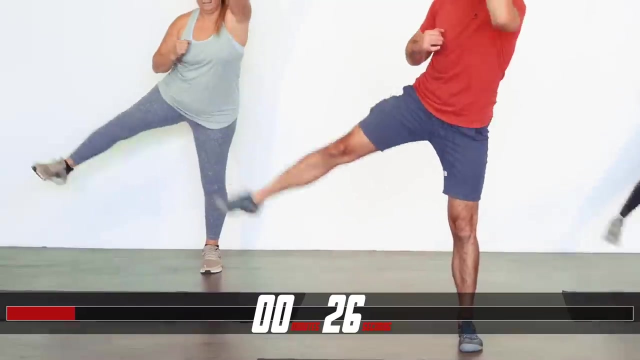 We're going to start with the first exercise of 30 seconds and it's going to be a side lift with an upper cut, left leg, right leg, left, arm three. we got this two and one off. we go. so getting nice, breathing deep, core, nice and tight, and you're gonna feel that tension in the left leg. it feels good, you don't. 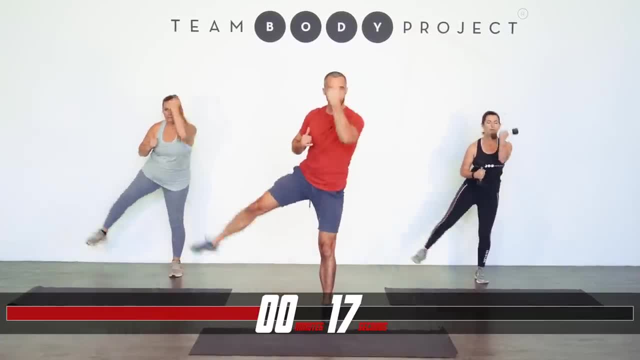 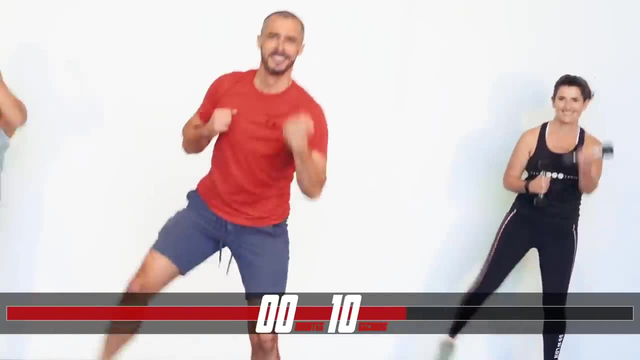 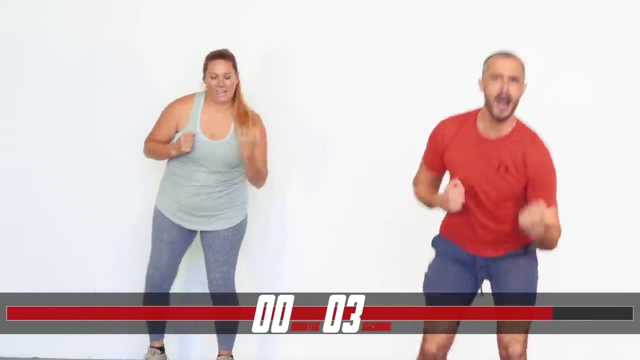 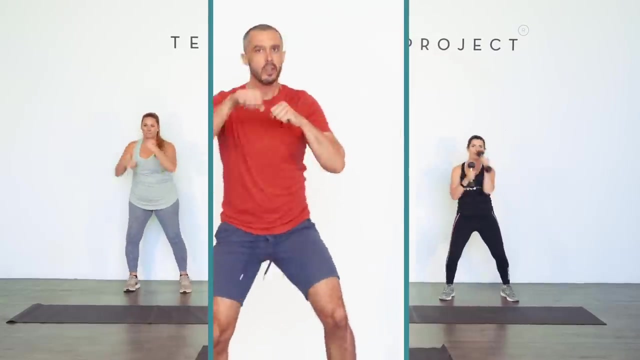 have to dip. you can just be steady. it's your choice and your workout. 30 seconds of fun- well, this might be stretching it a bit, but keep working through. core, strong eyes ahead, shoulders, proud, three, two, one and we're gonna punch, punch light. you can punch hard when you can see harsh. 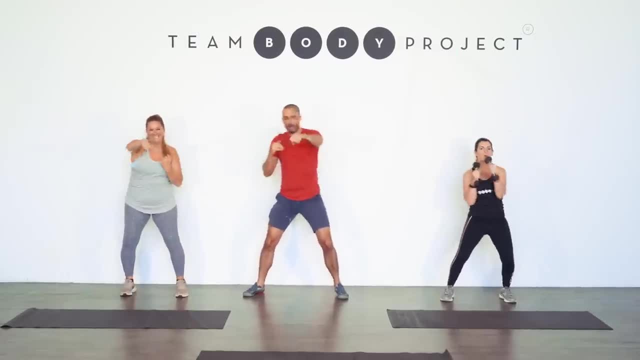 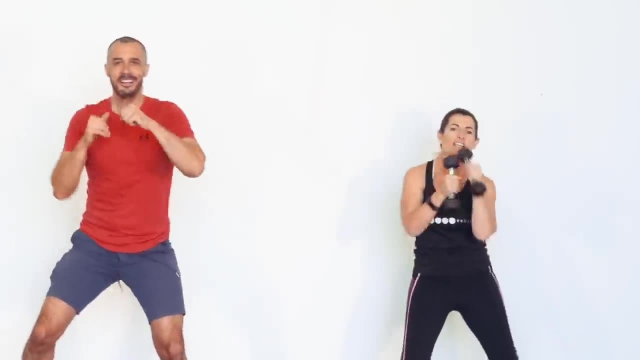 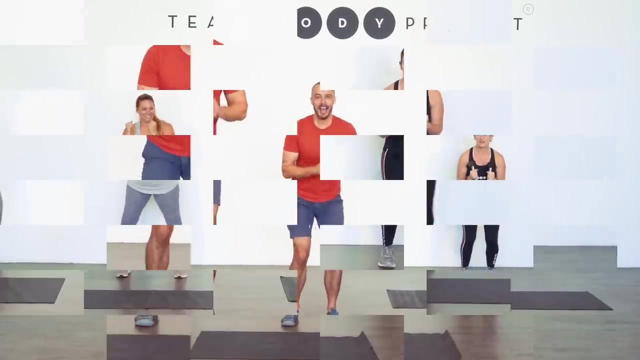 has got the weights. we're feeling good. you ready to do that again? which leg did you do? right leg out or right leg under tension? it's a good job. we got tash three, two and one, so here we go. so again, we don't need to dip. 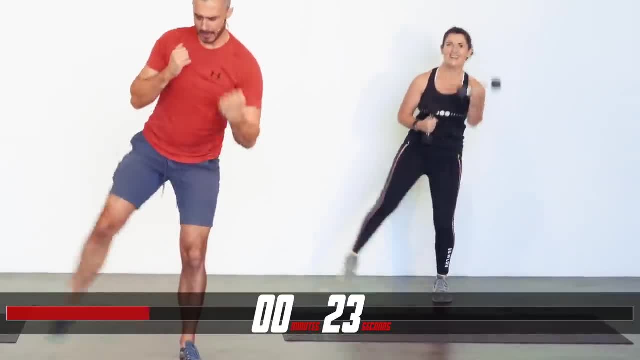 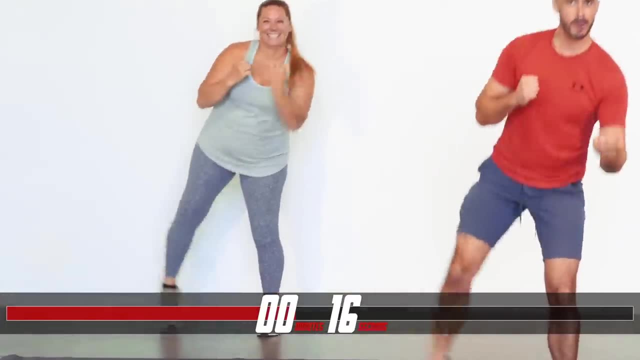 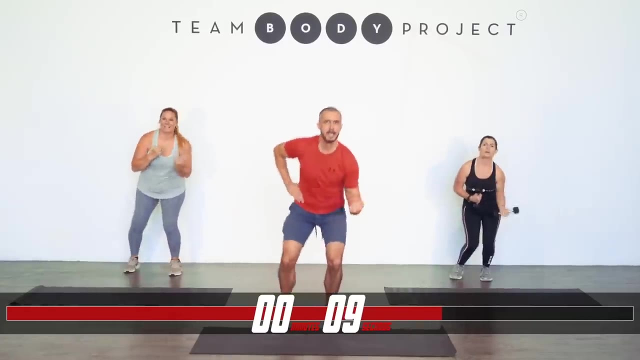 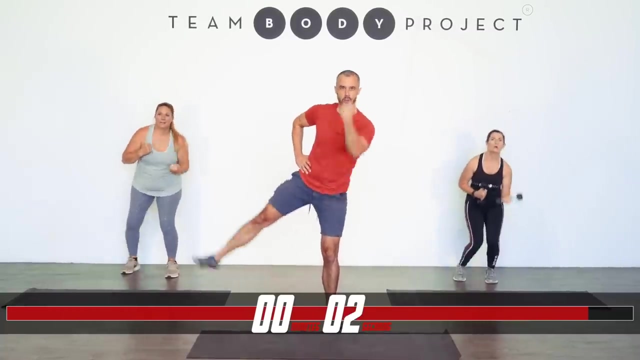 you'll feel that beautiful burn in the legs. you got it. don't hit yourself in the face. rule number one: a body, project, core, strong shoulders, proud, working through. stay focused. you can just stand. you could stop. just be here. all is good. three, two, one and march, and you can. 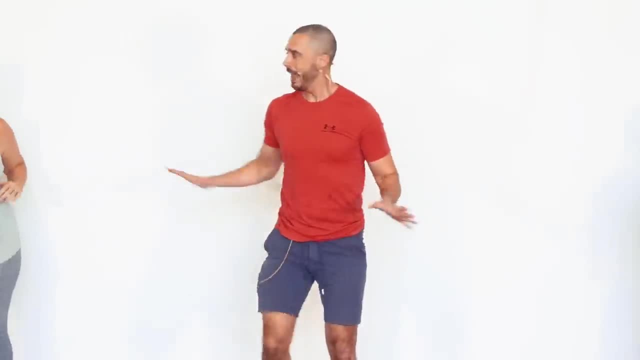 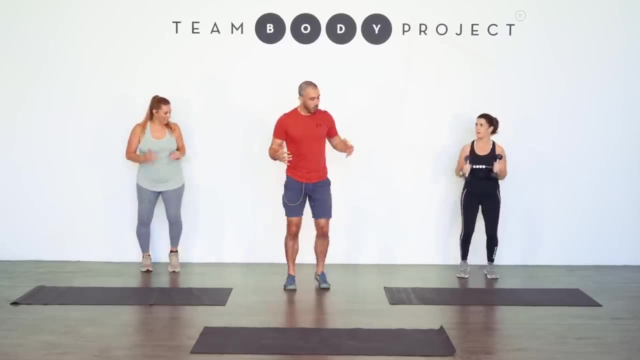 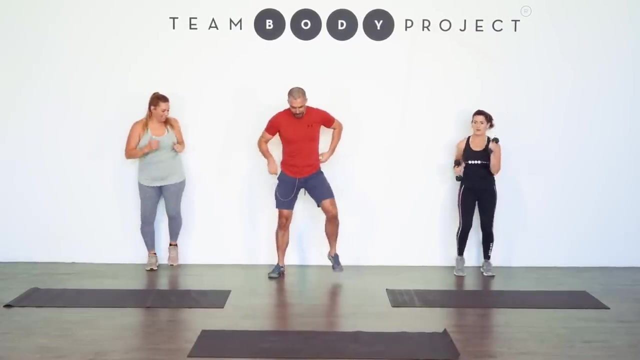 march hard or you can just march now. i'm not forgetting about the other side, but we're gonna do the other side in a minute. we're gonna now do a box step with a punch high and a punch low. you'll see when we go. you feeling ready. start from here: three, two, one step, step, step, step, step, step, step. 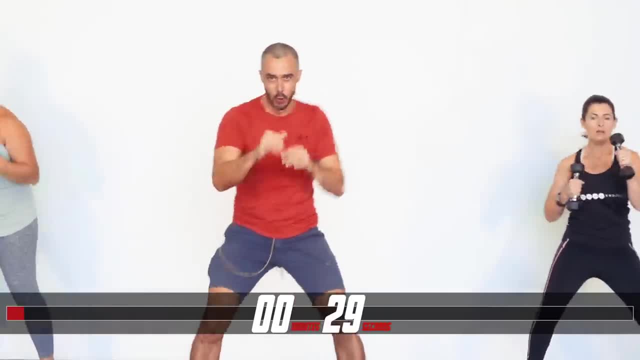 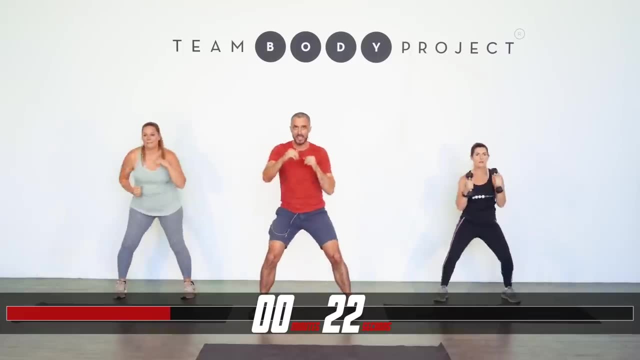 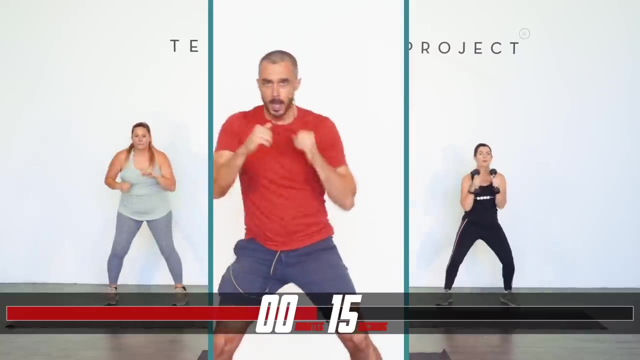 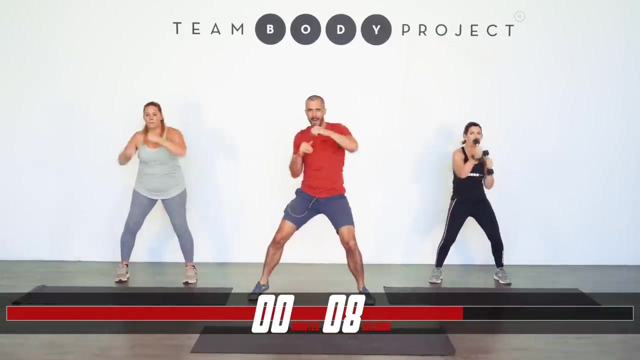 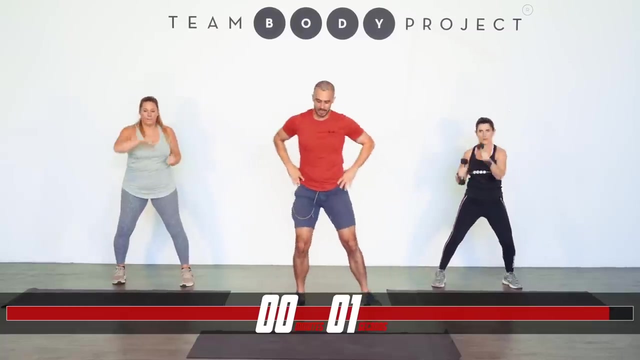 punch, punch, punch high. so feel that joy to be moving feels good. look at what your body can do. isn't it amazing everything in life comes through the body. come on, work, work, work, three, two, one and step. so we're gonna step out and again. you wanna go hard? you can step low and fast. 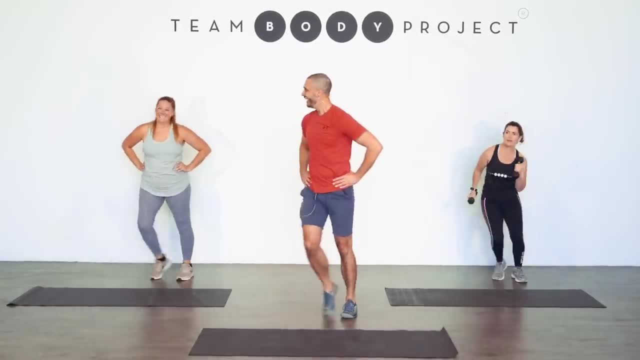 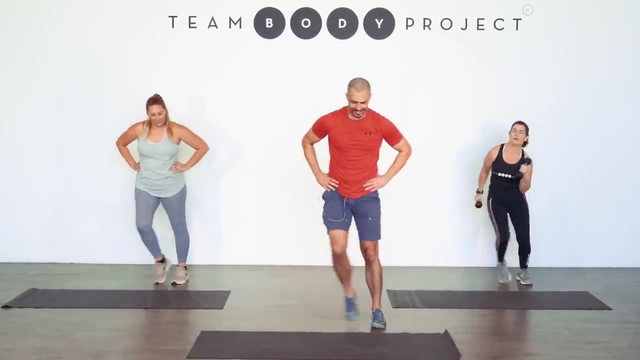 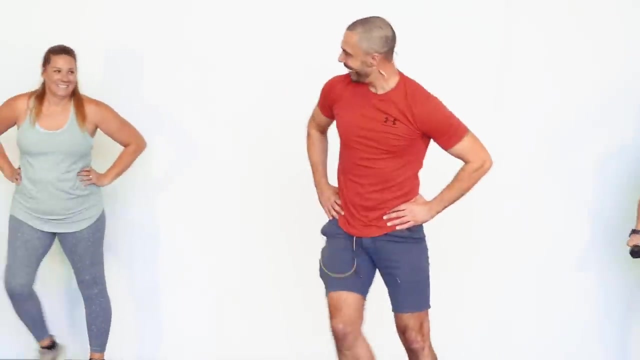 or you can just chill. it's hard and it looks that one, isn't it? it's a nice, nice, clean move that you really put some energy into which i love again. i use the word love somewhat lightly. three: we ready to go again. two and one step, step punch. 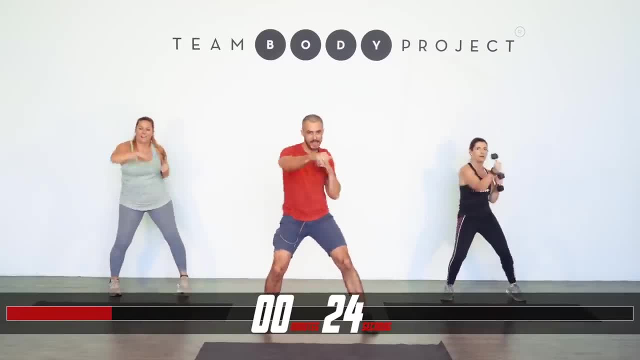 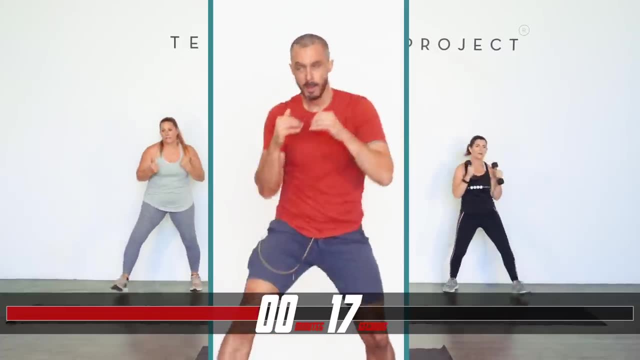 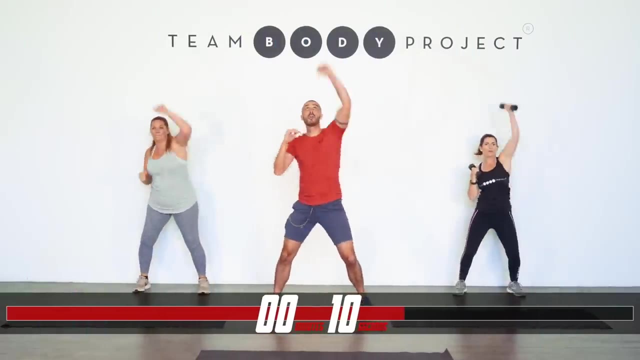 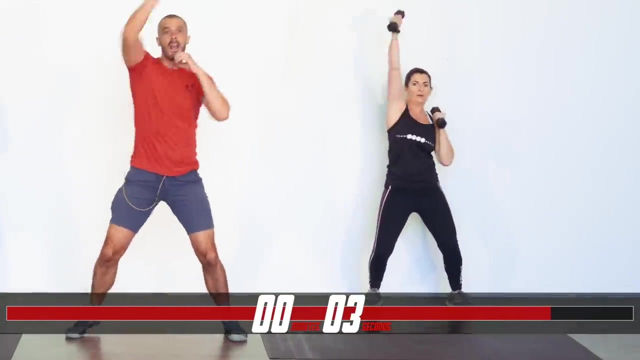 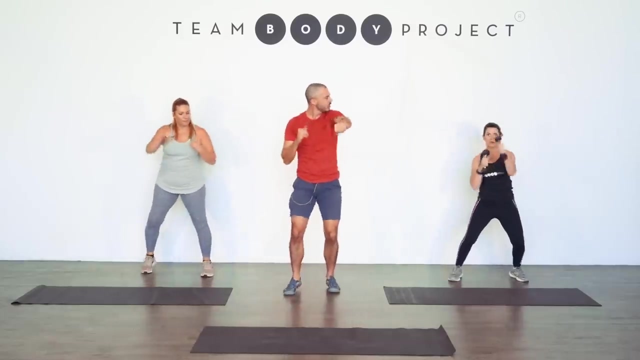 punch your best. your work, eyes ahead, cross, drop, pause whenever you have to. it's your session, even if you march the whole way through. that's a win. do your thing. three, two and one, and we're back on the light punches again. We're just gonna mix between those three. Fire it up. 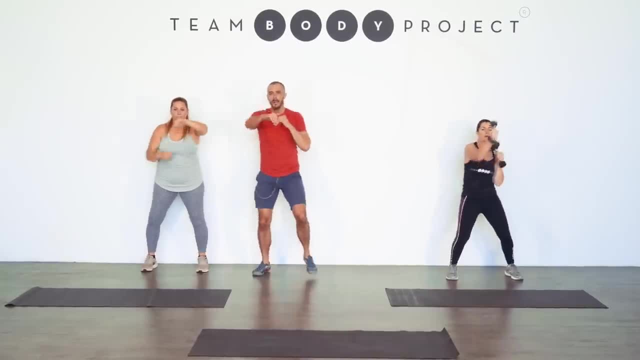 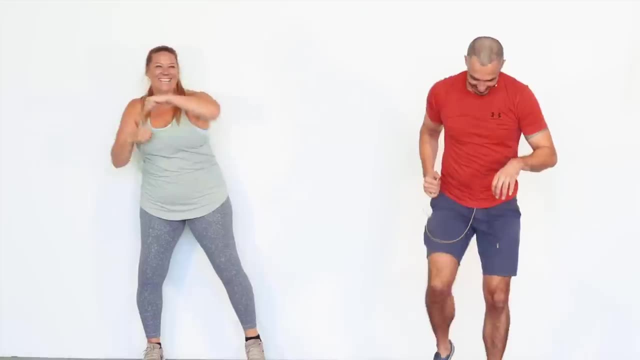 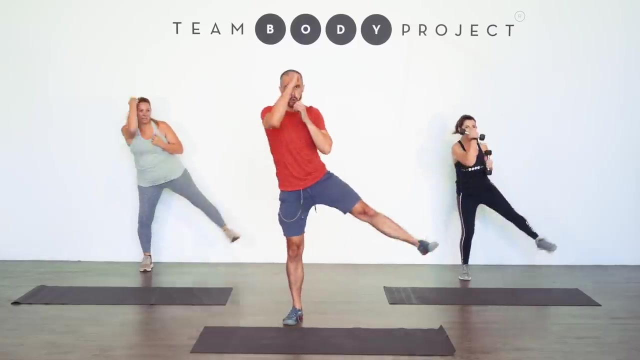 like Tash. So we're gonna do the other side. I'm gonna check, Kristen, which side are we doing now? Which leg? The other side? I'm pleased we got Kristen Three, two and one To that core strong. again, Your range is fine. Whatever your range. 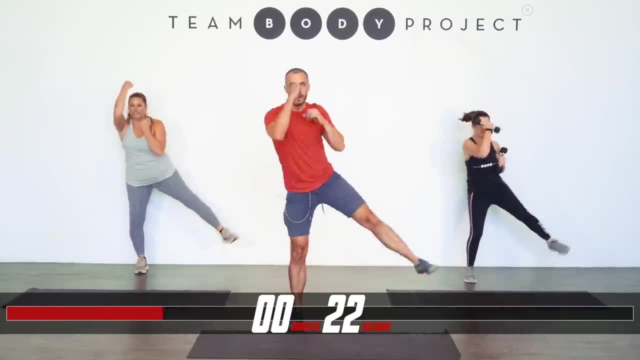 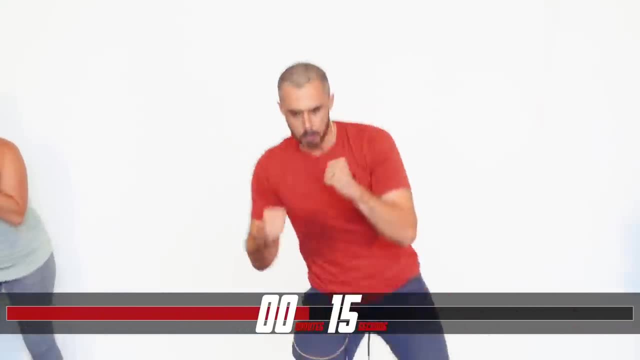 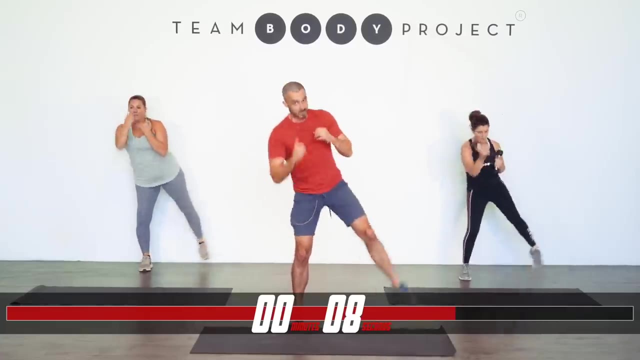 is Just do your thing, Working through, Remembering how spectacular your body is to be able to do this. It's beating your heart, It's oxygenating your lungs, It's feeding your muscles. Movement is the best thing in the world. We're doing it. 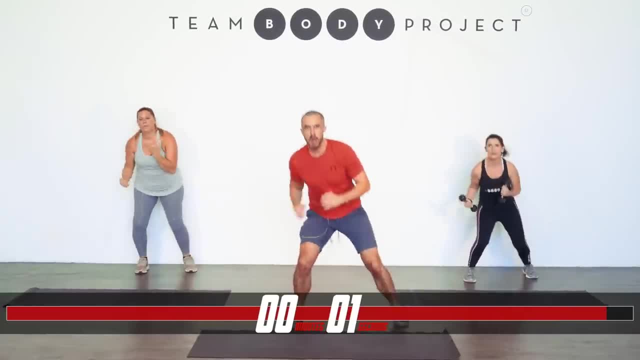 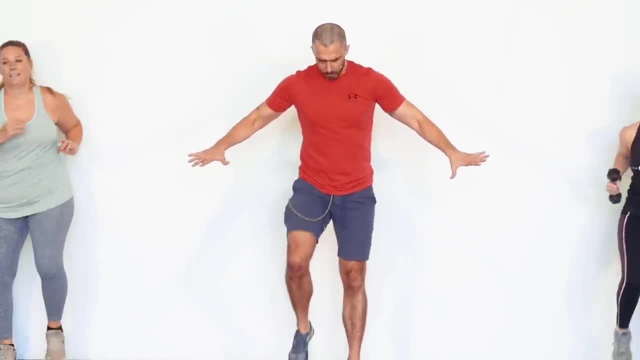 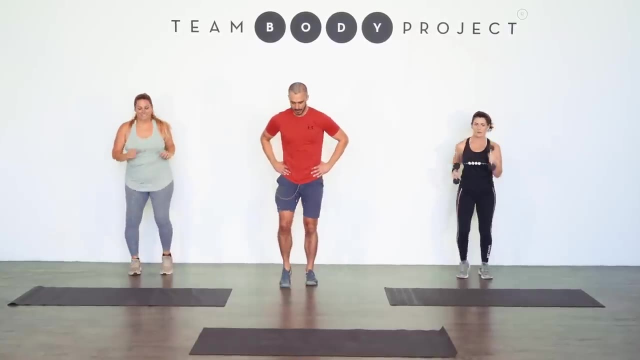 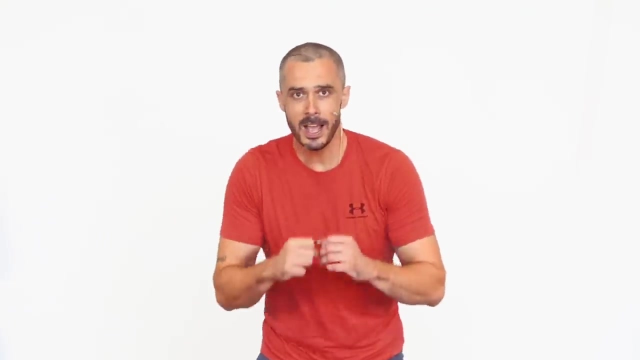 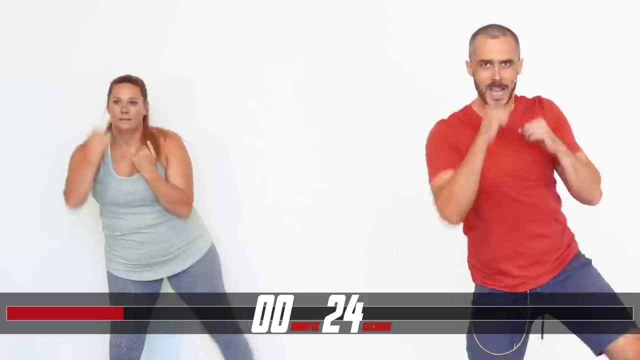 right now. That's why we're winning Three, two and one and march. Breathe, You can pump, You can recover Going again Right arm, left leg, The other side, Same side. Three, two and one and off we go. It's really tuning in. now Feels good. 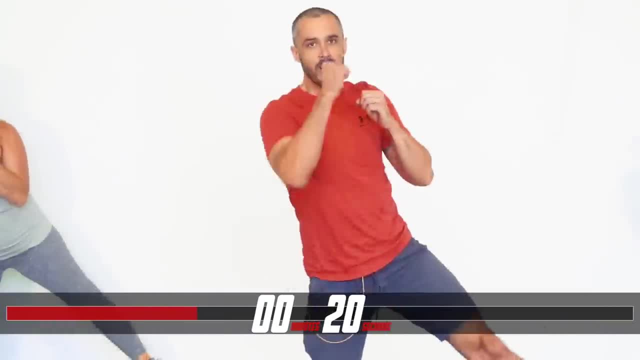 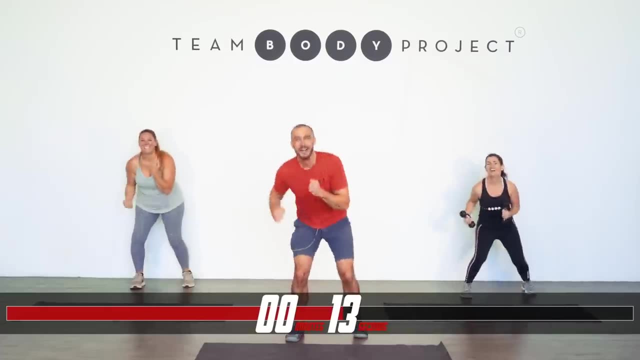 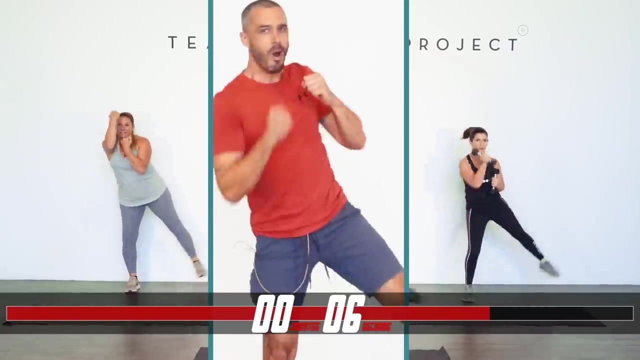 doesn't it? I'm not sure Kristen believes me yet, But she's new, She'll learn. It does feel good. At least we convince ourselves that it does. Core: strong Engage, Working on Working through. Come on, Here we go, Here we go. 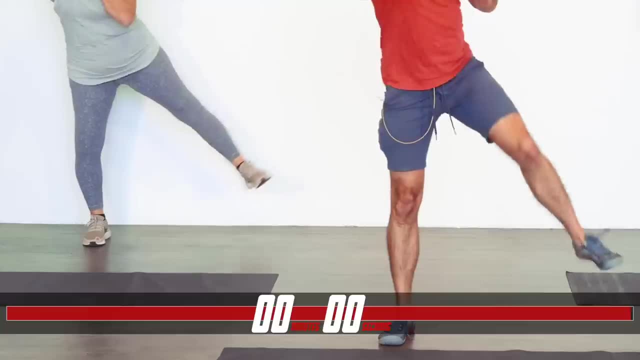 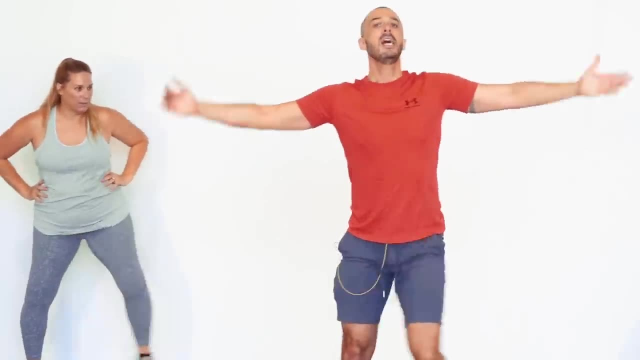 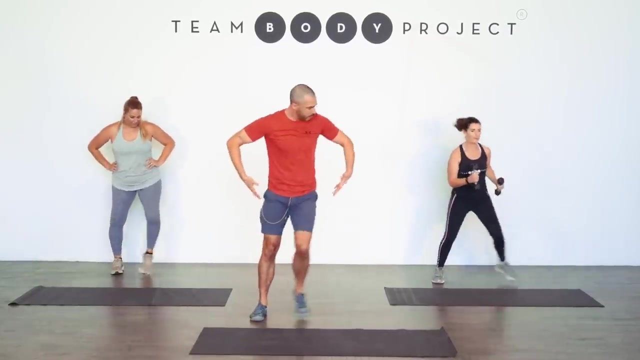 Into the side step in three, two and one. And still we move. But you can pause completely, That's still winning. Just don't leave Big wins so far. Next exercise: come in now. We're gonna keep these steps. What we're gonna do? a chest clap and shoulder. 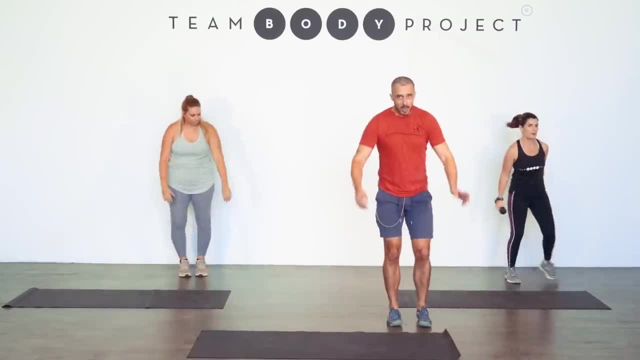 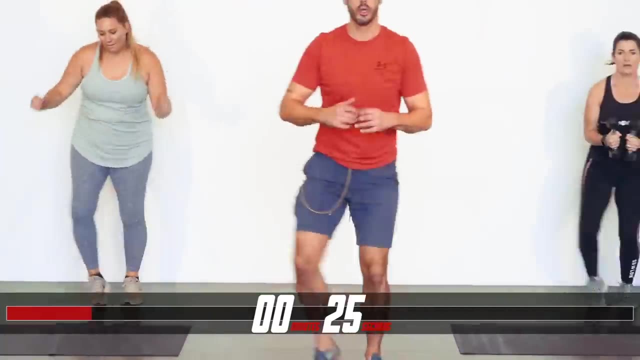 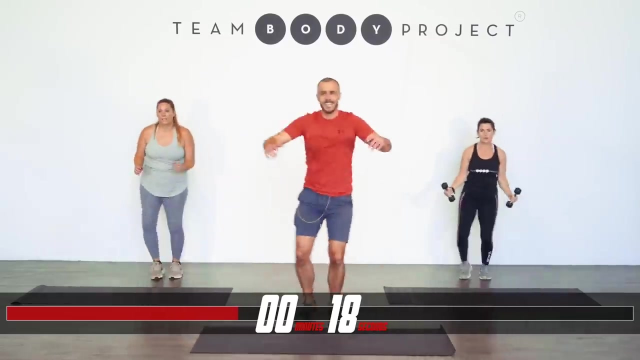 clap We ready for that. Coming left to this side: three, Two, one Step, step and higher. Now this feels good: Core, strong Shoulders, proud Breathing through, Digging deep. This is a celebration today. There's no punishment that goes on here. We love it when I'm. 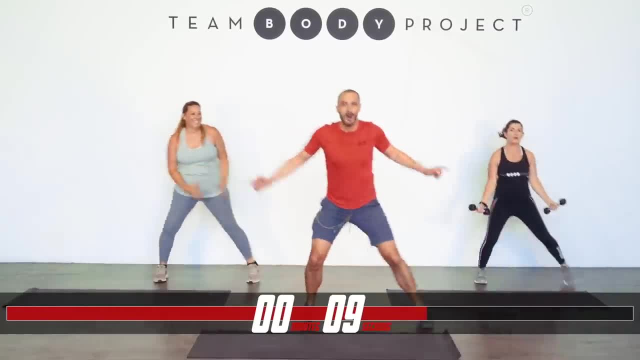 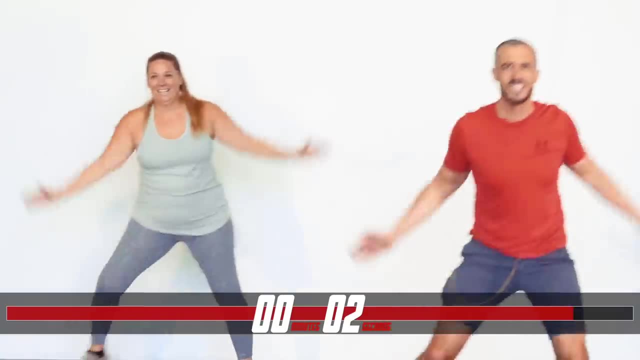 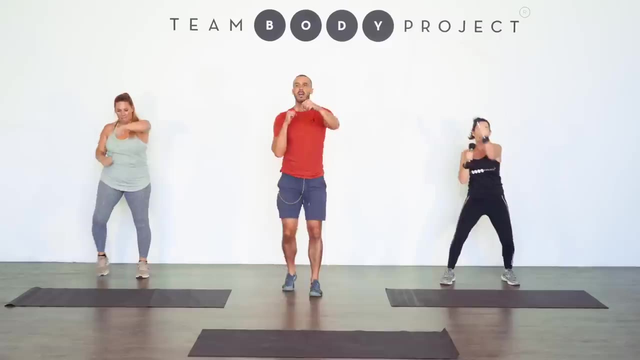 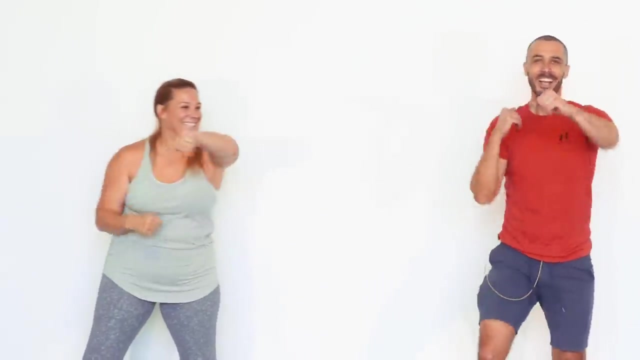 messing it up. I am. I'm getting it right now. It's hard Into the punches. next, Three, two and one, And again you can breathe and recover however you want to. You like that move? Yes, It's a good one, wasn't it? If I got it right. 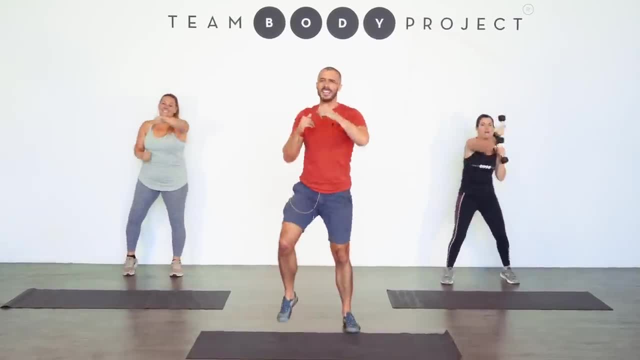 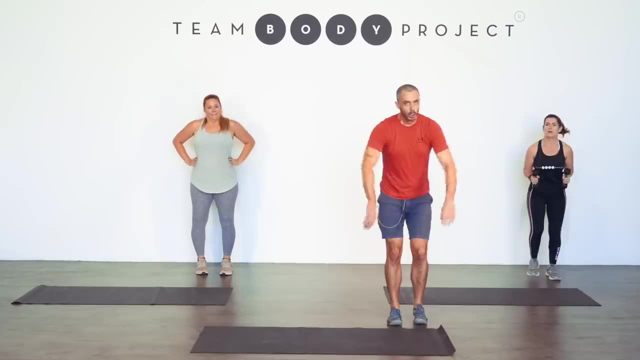 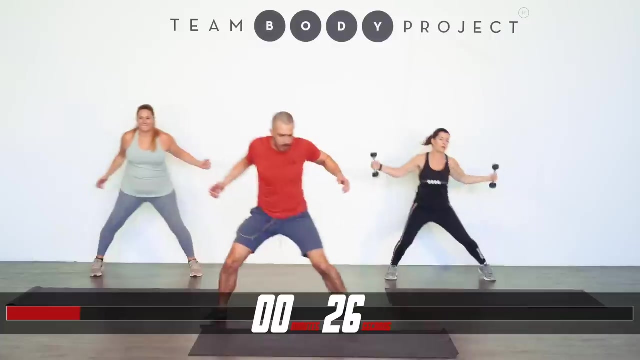 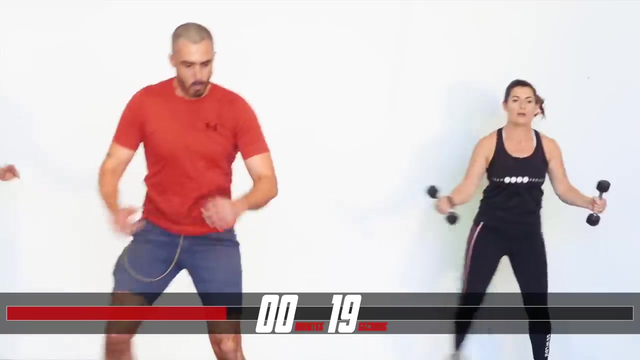 Quiet And go Okay. Three Break whenever you have to. team Two and one Ha Strong Power, Resilience. It's all going on here. That's what's needed to finish a session like this. in your own way, in your own time. Feel them muscles. 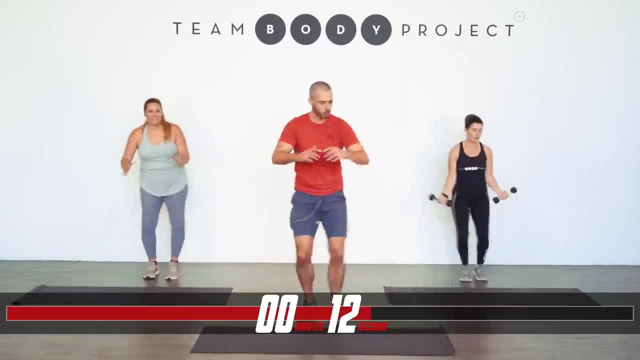 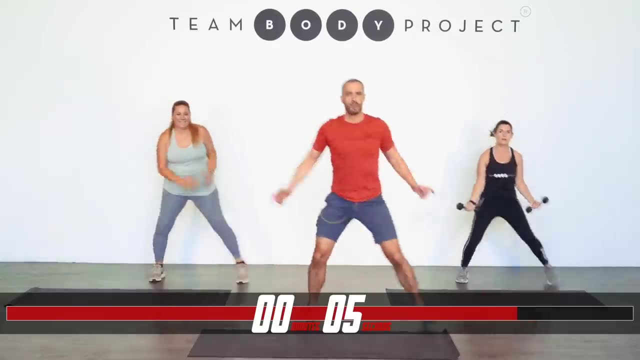 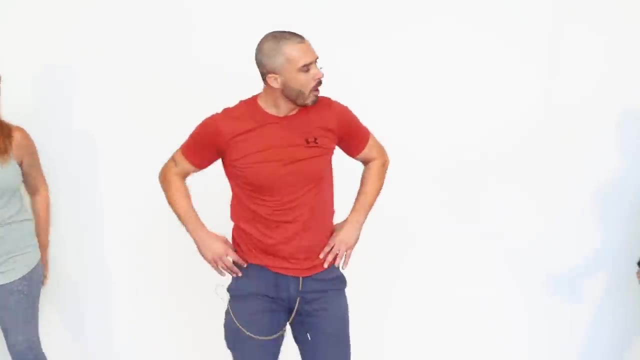 working, Feels good, Sure, Body Core strong. I got that one wrong again. I'm really not doing this very well anymore. It's okay. Three, two and one. Well, we got the steps. March, march, It doesn't really matter, We're just going to move as we see fit. 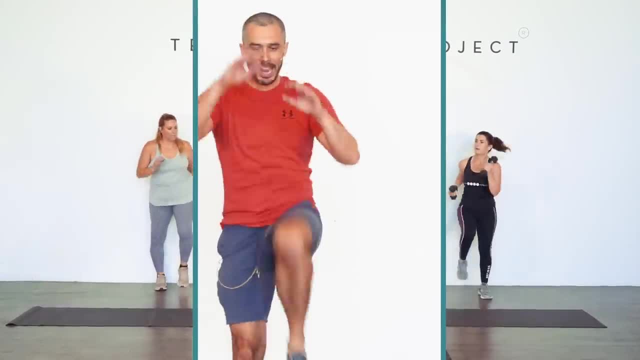 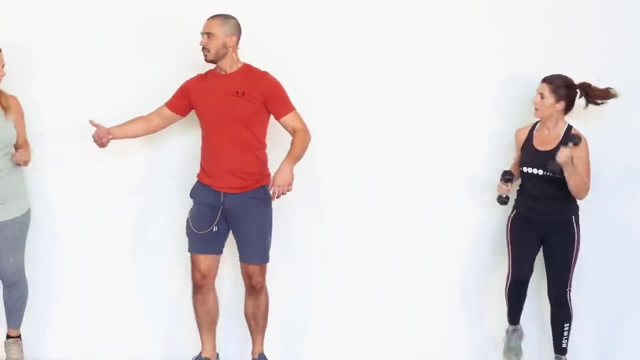 So next up, keep going. I'm going to demonstrate. We've got a high knee hook hook, High knee hook, hook And we do the other knee the second time. through Making sense, How are you feeling? Double thumbs up. 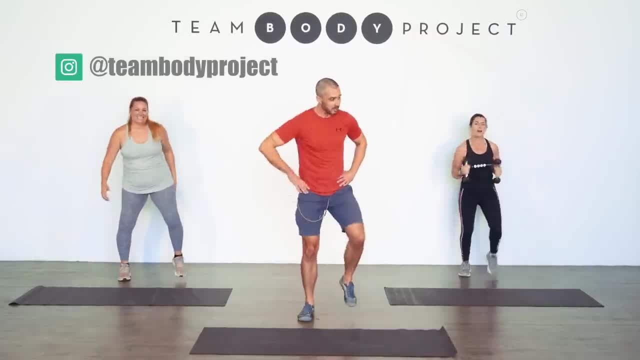 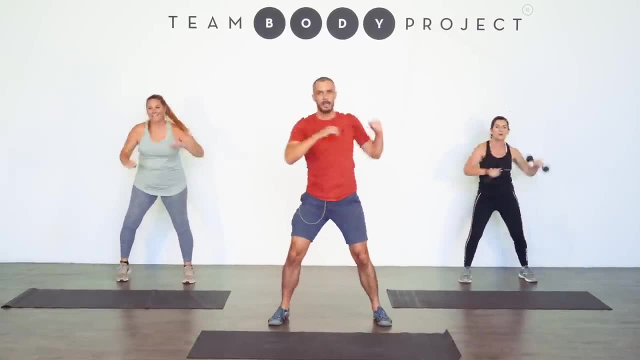 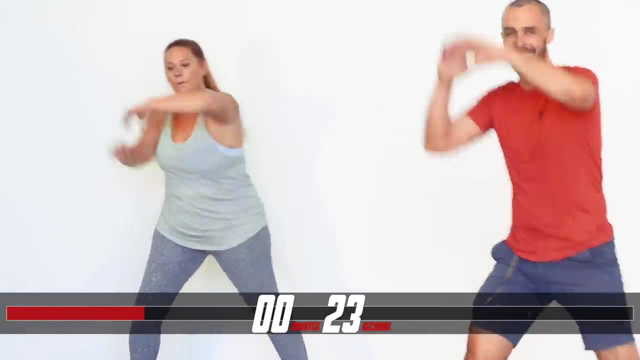 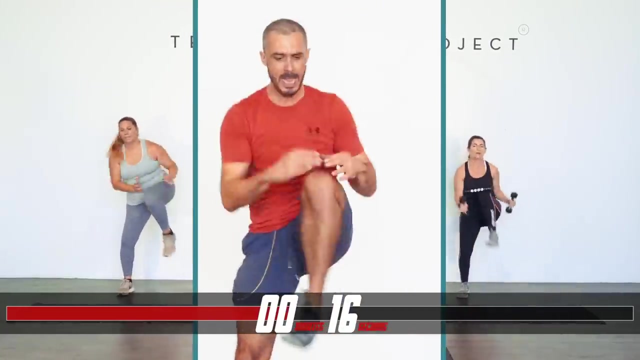 That's twice as good as one thumbs up Three, two and one. Lots of energy here. Your speed remember, not our speed. Come on, Feel it flow, Feel it work, Feel the goodness in the movements, every movement, This movement. 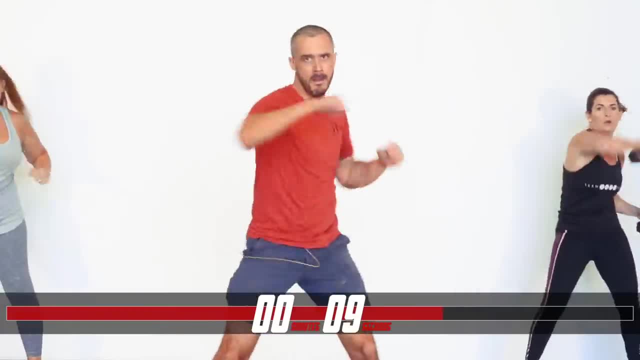 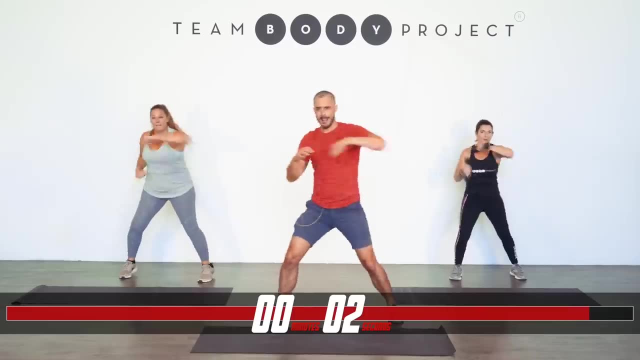 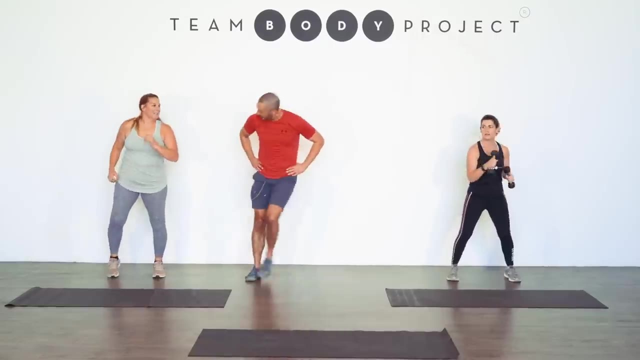 And this one, And this one. Get that adrenaline in now And suck it up and use it. Three, Two, One. What have we got? Steps, Step, step. There we go. I can see you sucked the adrenaline up there, You did. 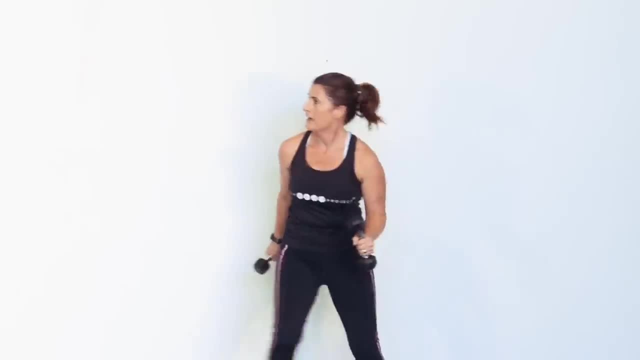 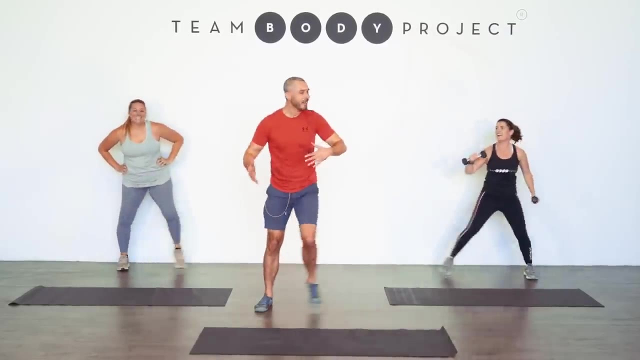 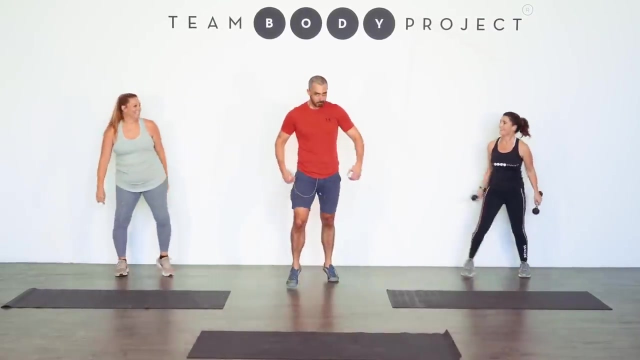 didn't you? You got it in. You got to be quick there. Tosh, Just don't show me up too much. that's all. When I come back, slow down and then speed up again when I've gone Right. We've got the right knee this time. The other one, Three, two, one. 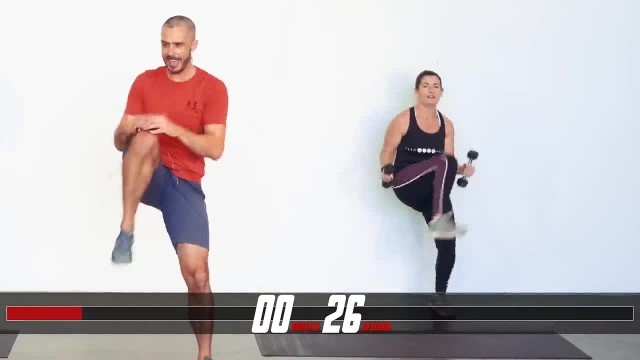 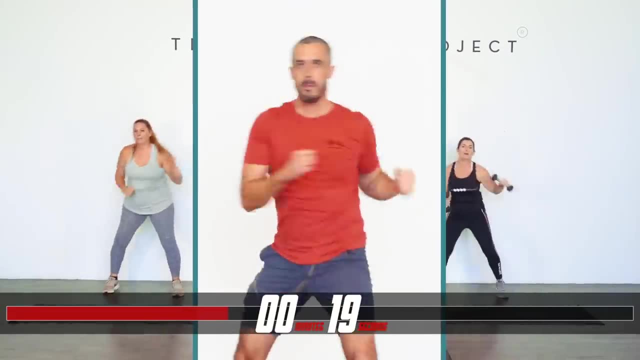 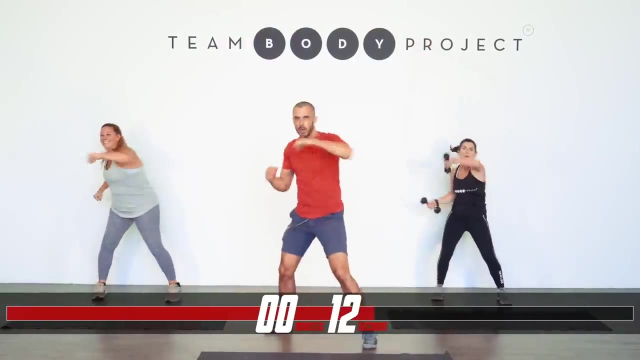 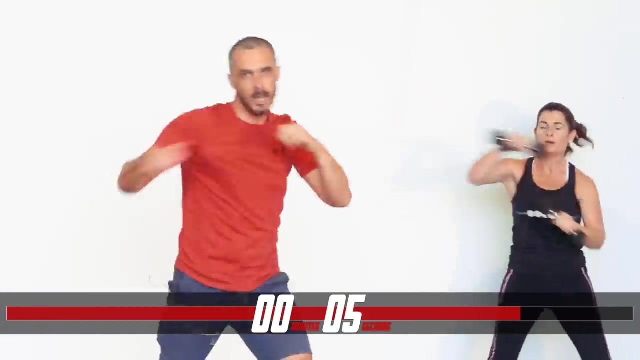 Get that energy in. I love this Multi-level. Do your thing, Don't have to keep up with me, don't have to keep up with Tosh or Kristen. Do your thing. Core strong eyes ahead. Three, two, one. 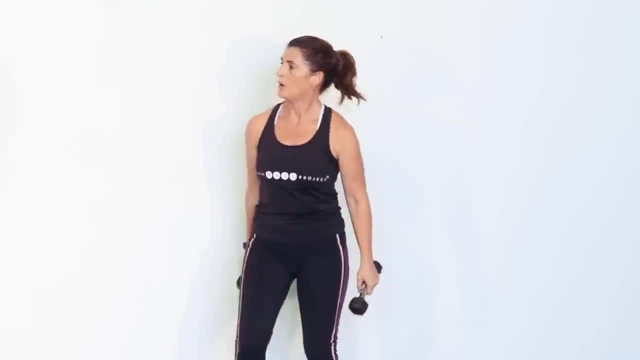 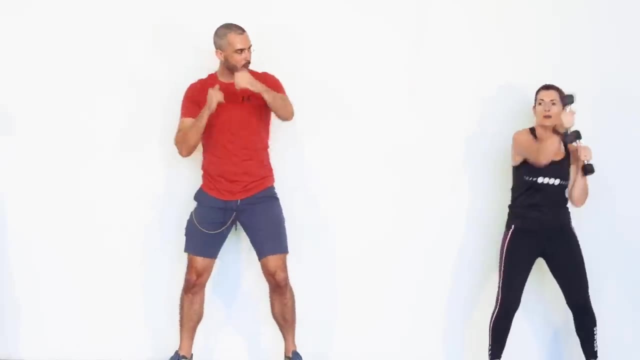 And breathe. Are we marching? Are we stepping? Are we punching? You reckon punch. Let's go Nice and light As light as you want to. So we're going to come into the step back oblique. We're just going to recover ourselves for a second, or you can push with Tosh. 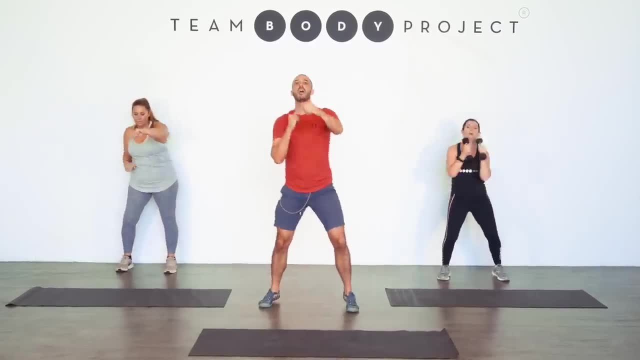 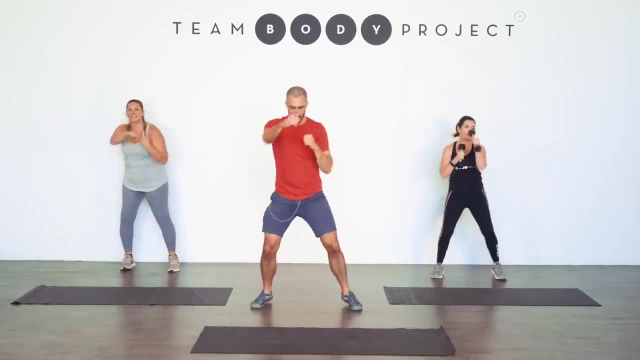 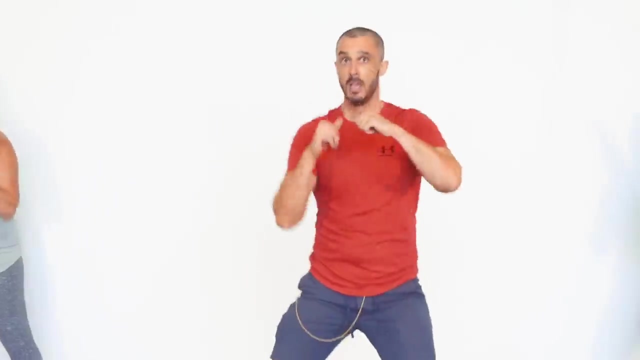 But what I want to say? we're all on our own journey, Every one of us. The only similarity between us all is that our bodies are magnificent. They're part of us, and moving them right now is important. That's exactly what your body wants and deserves. You're a winner and a warrior. 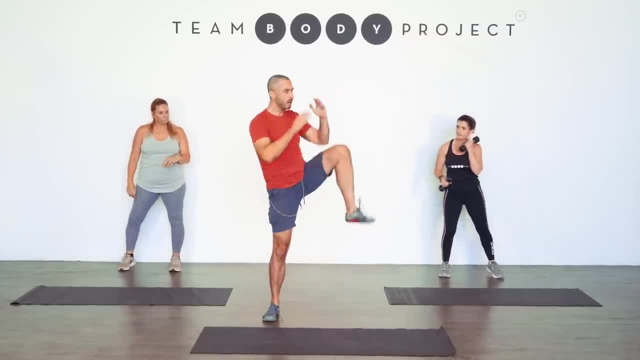 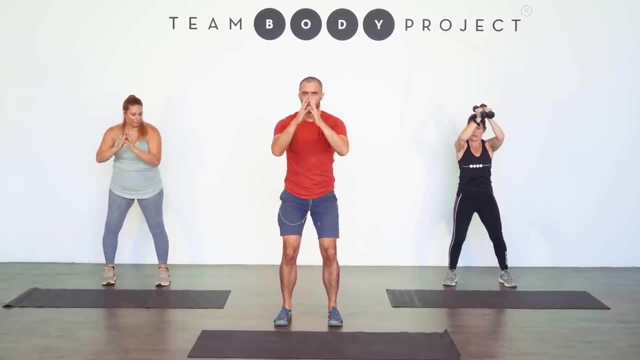 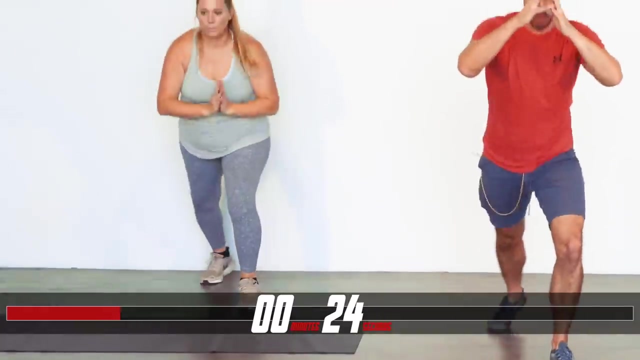 Remember that We've got the step back oblique crunch. You can have the hands starting here. You can keep them low. It's up to you. I'm feeling this: Three, two, one. You don't need to lunge down, You can just step This right now. 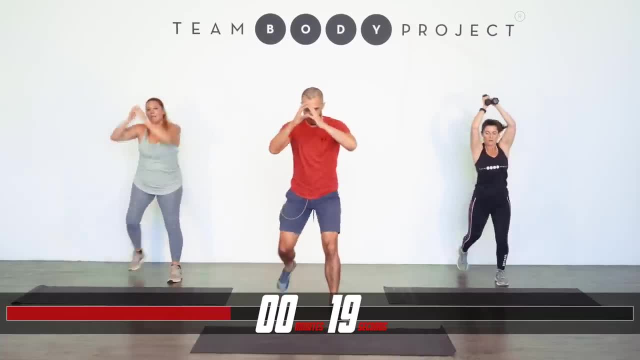 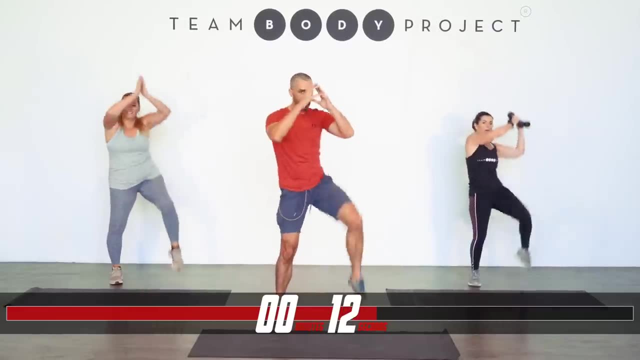 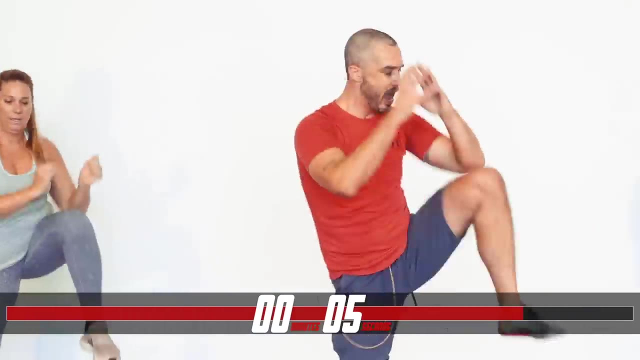 as that sweat's pouring off. this is waterfalls of progress. right now You feel their muscles. That's change juice. That's progress coming at you fast, coming at you hard, because you're earning it with every movement, even in the march, even in. 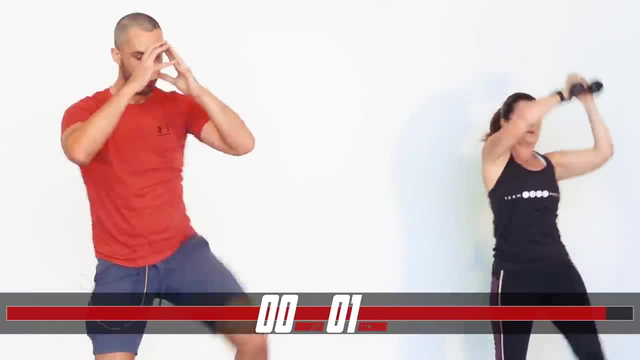 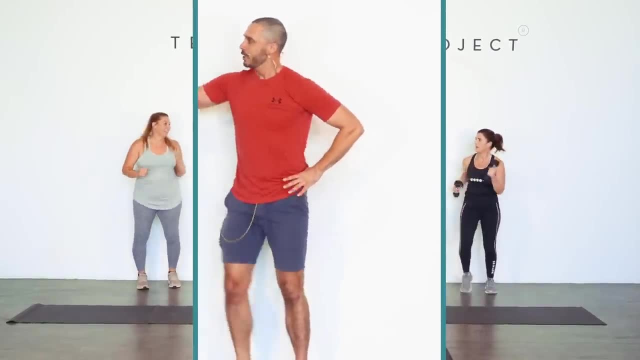 the pause because you're here. The habit's coming: Three, two and one and we bring that into a march. I like that one so much. we're going to do that side again. Only one thumbs up. that time We dropped one thumb. You can get that in there. Come on, You're. 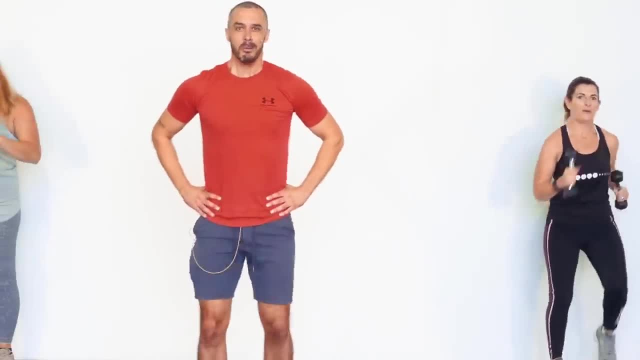 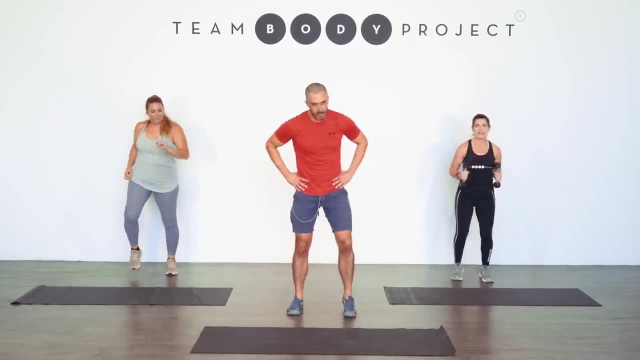 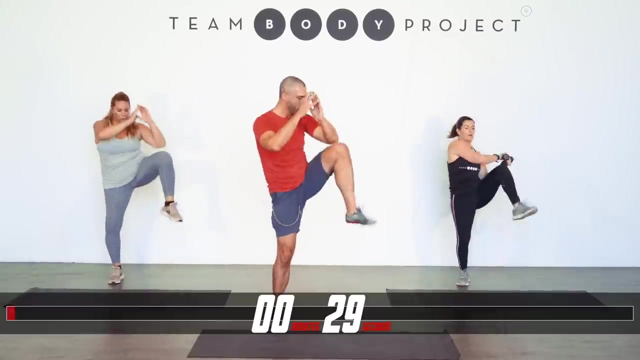 thumb Can't say I'll blame you. I'm kind of feeling that way too Okay, which leg did we do? Right leg back Three, two, one. So we're going pretty quick. We're all feeling the benefit of that beautiful adrenaline, Focusing on your pace, your 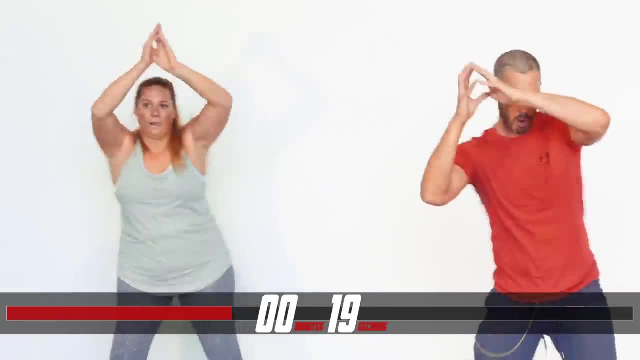 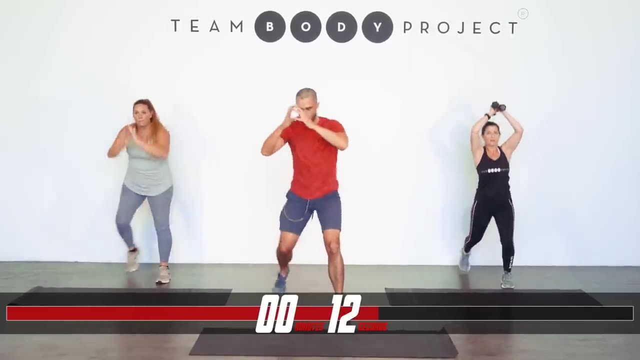 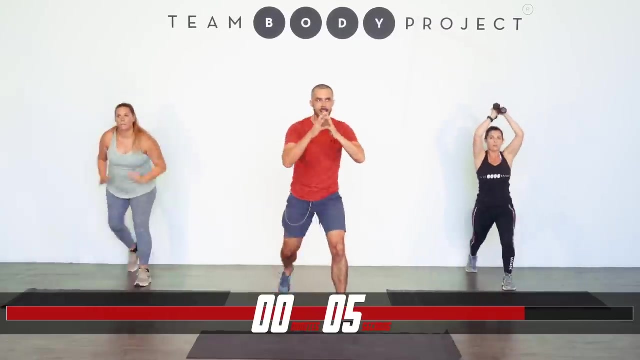 journey. All a win Every moment. This workout can be as advanced as you want, or it can be a starter workout. It's your choice. It's your body. You chose to be here And that's why you've got my respect. Three, two and one. Let's punch it out. 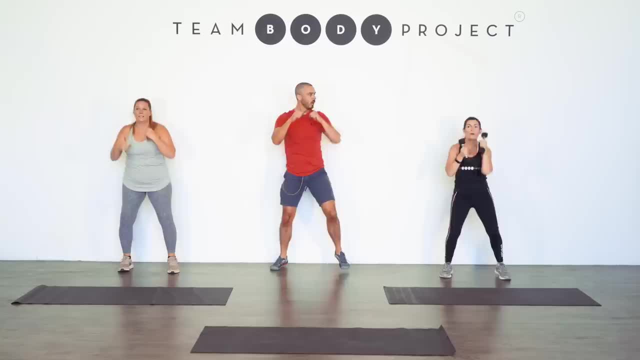 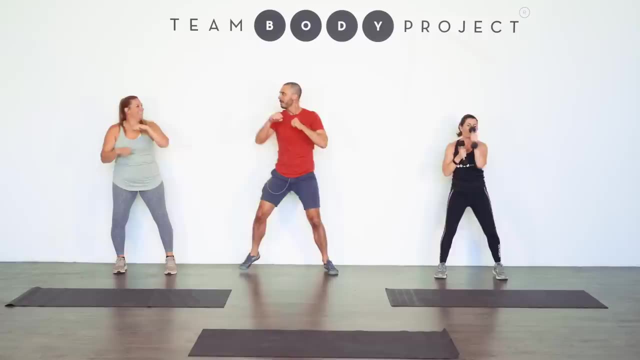 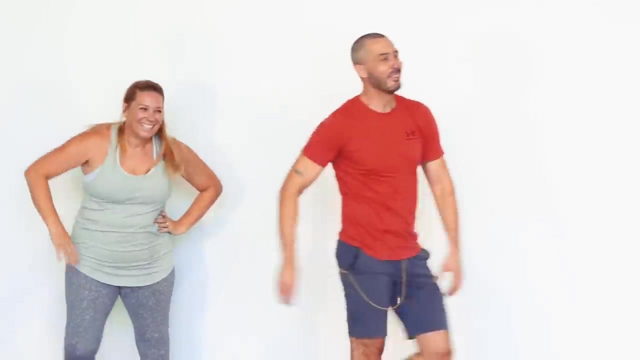 Let's punch it out. I'm feeling that Are you? It's tough. Breathe, Breathe, Pause, if you need to. Anytime, Kristen, Anytime, Anytime. That's good, That's good, I'll come with you. I was waiting for you to do that. I was thinking. 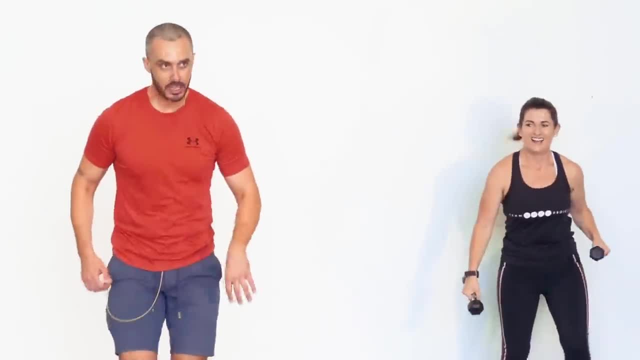 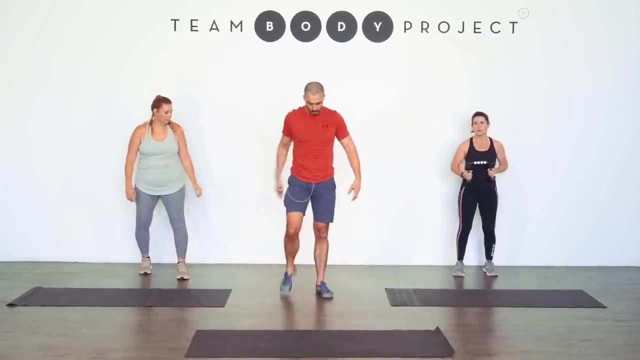 when is she going to pause? I need a pause, Right, okay. So next up, we've got the step out, touch and raise, Step right arm. In this one it's right arm. Step in and step out, touch and raise Three. two start with the feet together. Core strong One. 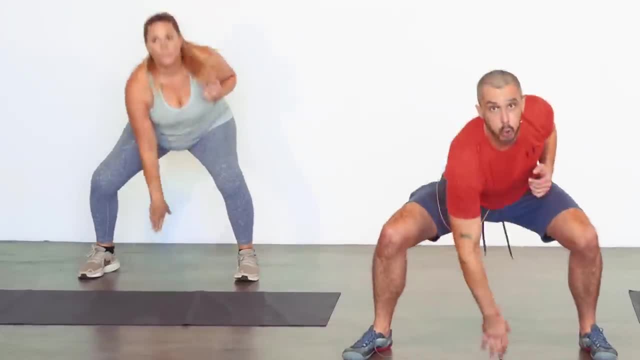 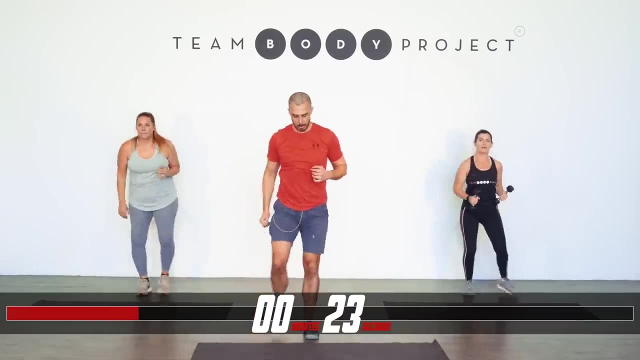 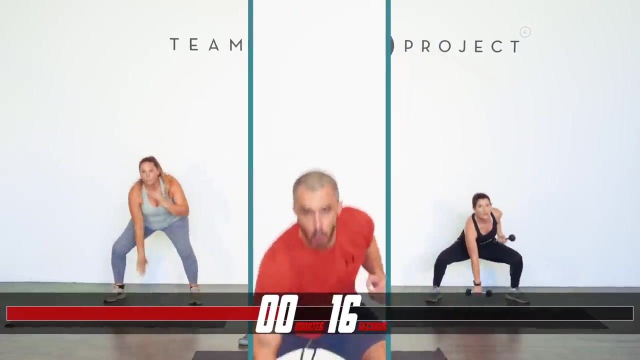 two and one Touch. raise Nice and high Reach, high Reach for the sky, but only go as low as you wish to Keep your shoulders proud. Look ahead, Find a point. Here we go. I love this Needs a little. 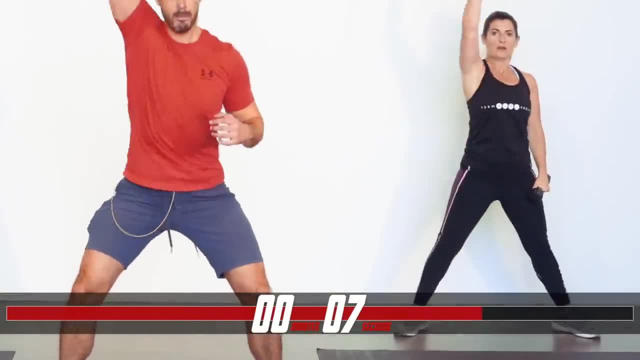 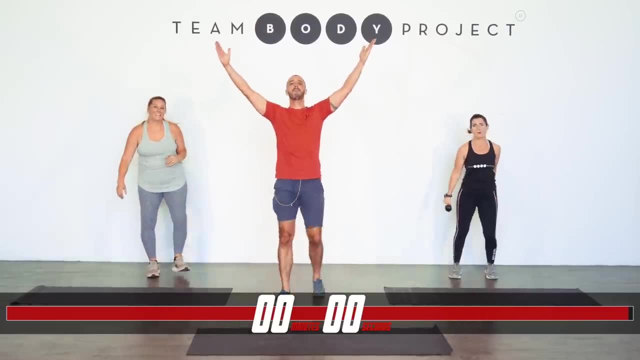 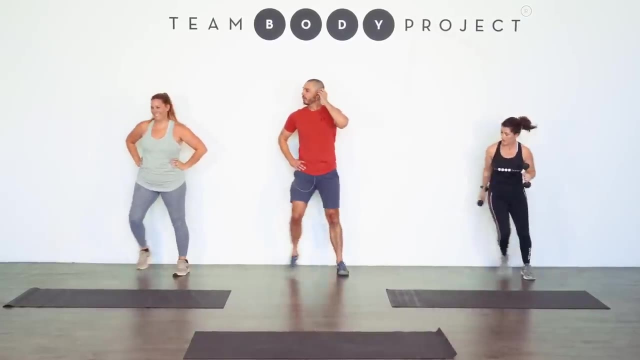 coordination here. It's okay if you're finding a little time to get this one right. Three, two, one: It's all about moving Breathe. Oh, we're stepping out. Let's do the step out. Let's do the step out, As I'm getting tired, I'm forgetting what we're doing a little bit. 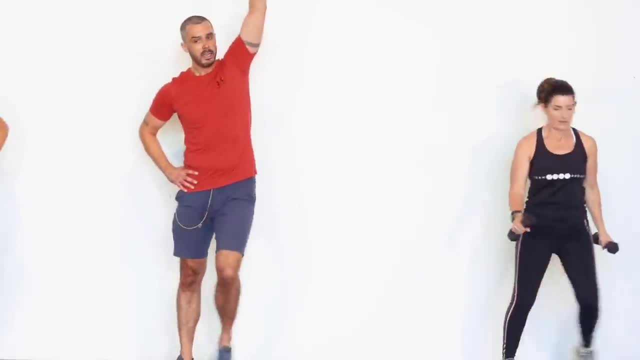 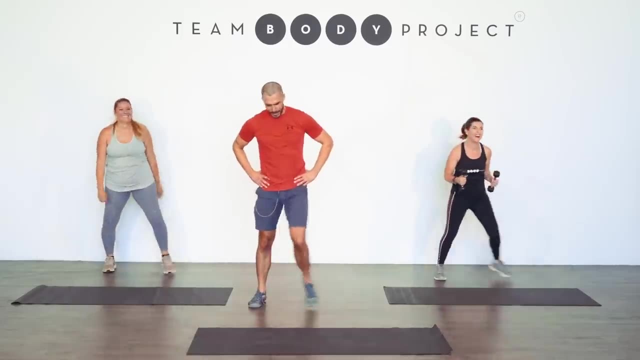 Okay, so we're going to do that again, except the left hand is reaching for the sky this time, Ready to go again. Tosh, How did I know you would be Three, two, one High. There we go. 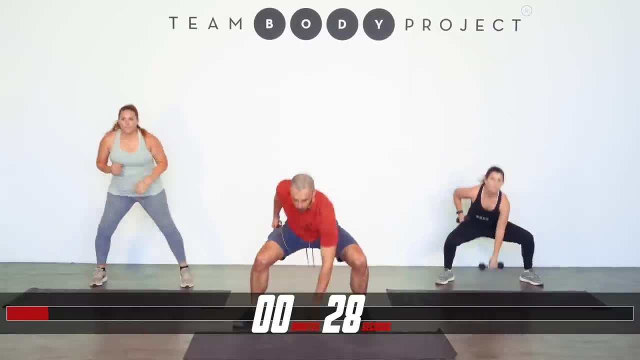 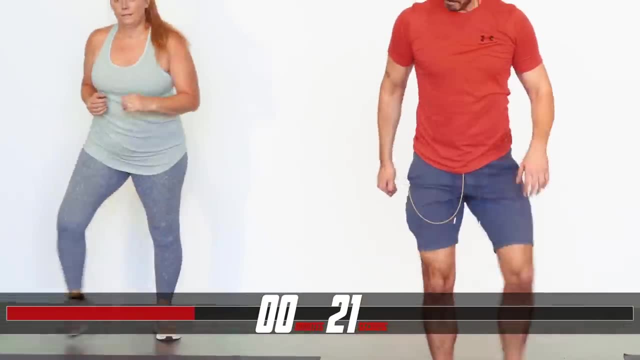 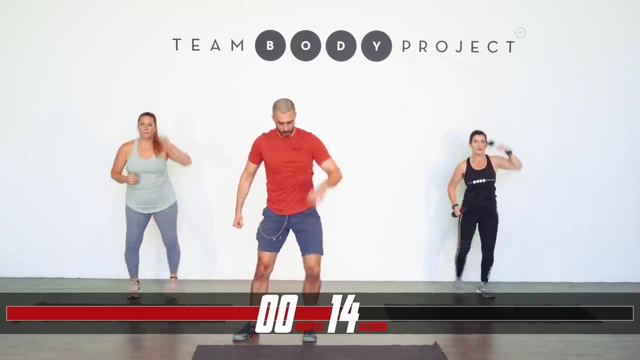 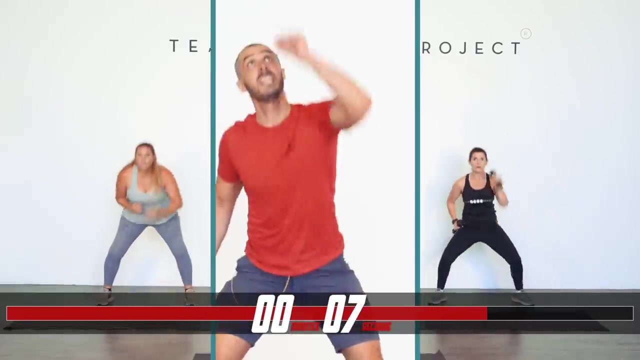 Reach high. Yes, There's the win. Grab it, It's yours. You're earning it with every second. There's nothing like moving. It's a celebration of what it is to be alive. That's what movement is. It's life. 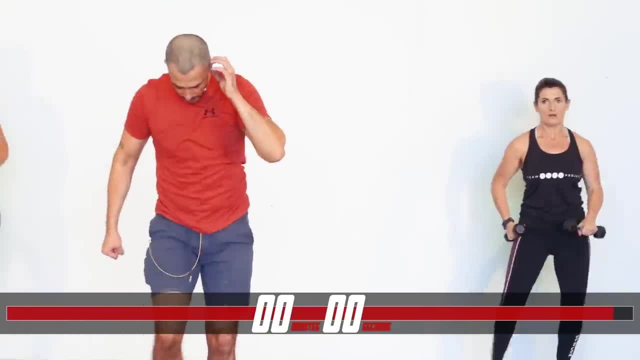 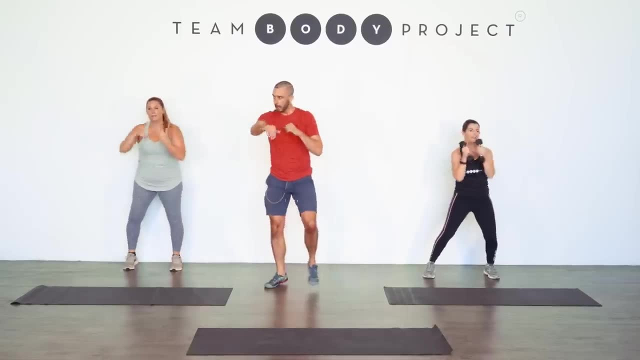 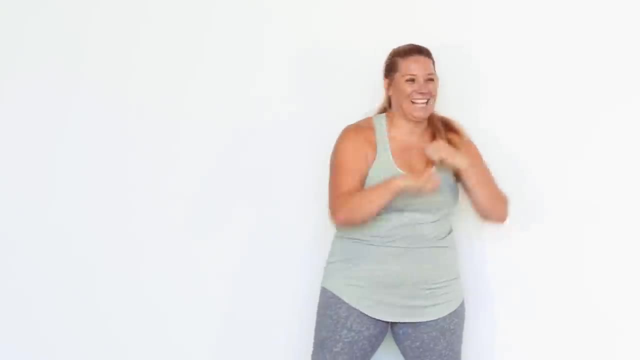 Three, two, one And one. Let's punch it out. And then we're going to do that other side on the step back oblique, which is the other side, Left side, stepping back. It's a real relief we've got Tasha, actually Three. 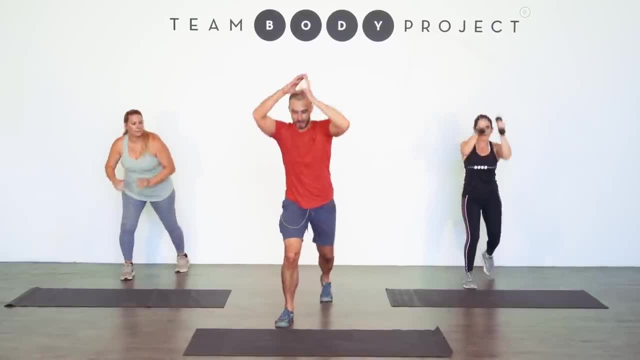 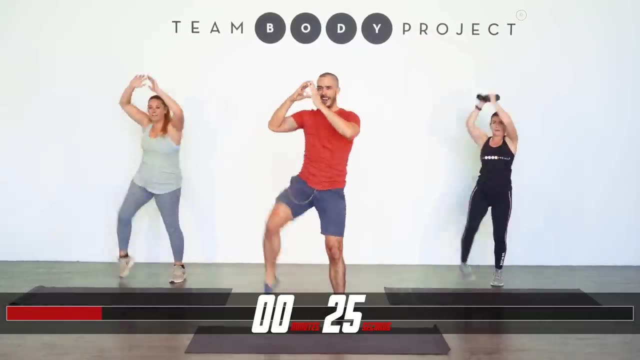 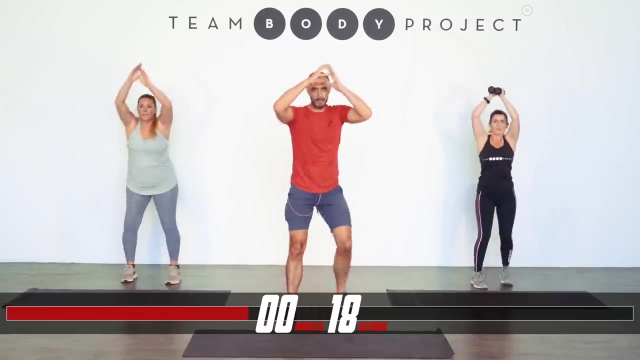 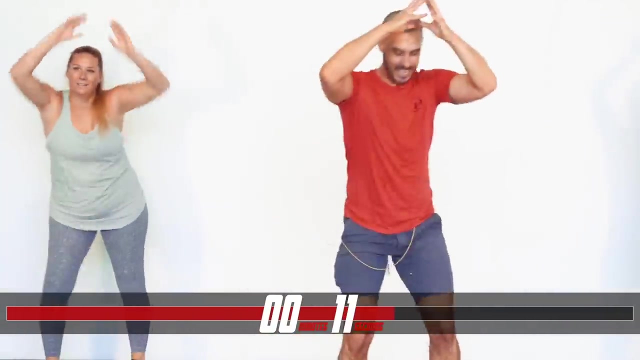 two, one Step back and up, Wherever you are with it. that's a win. There's a little coordination in this. today, I'm going to tell you the truth, I was up all night practicing because it's not my strong point, but it doesn't matter, As long as that body's moving, we're working out together. 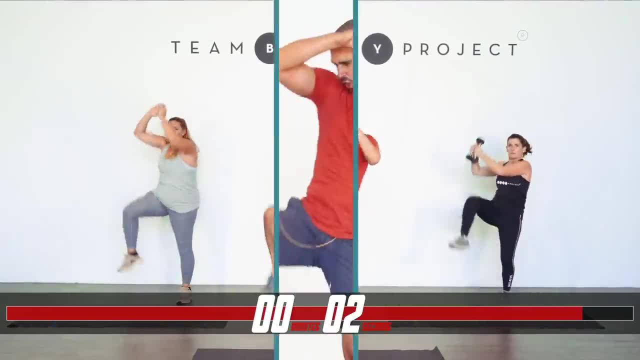 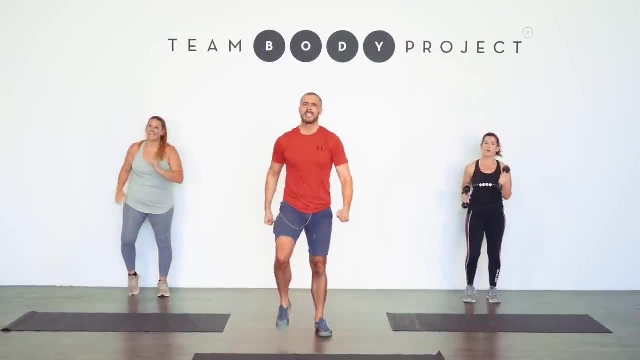 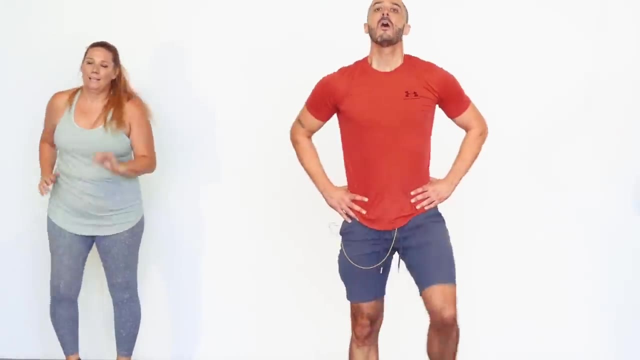 Three, two and one. Should we bring that into a march? Stay strong to it. Come on March as hard as you can. Suck it up now. Why did you press play? Why are you here? Remember that We're hitting. 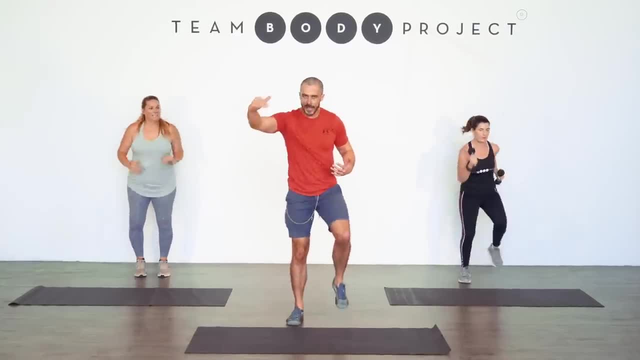 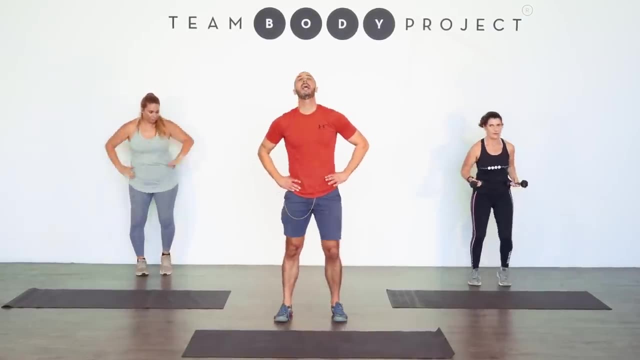 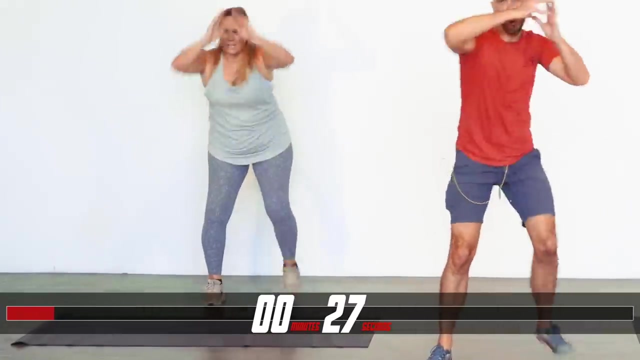 that tough point. now, That's where we've been over the top. It's coming down the other side. We're going to win. We're going to win Left back, isn't it? Three, two and one. Here we go, Push through. It's like a core, It's like a rock. It's strong. 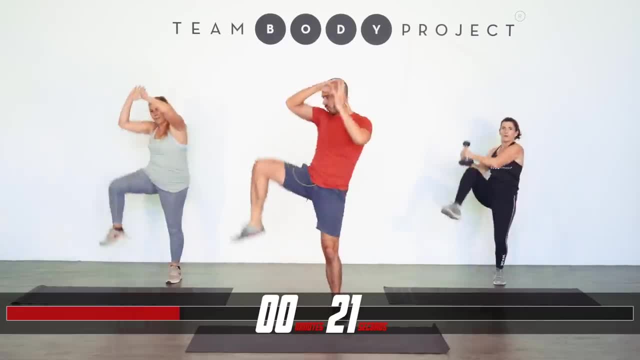 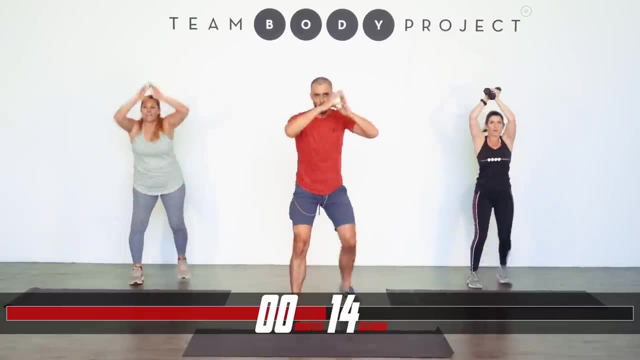 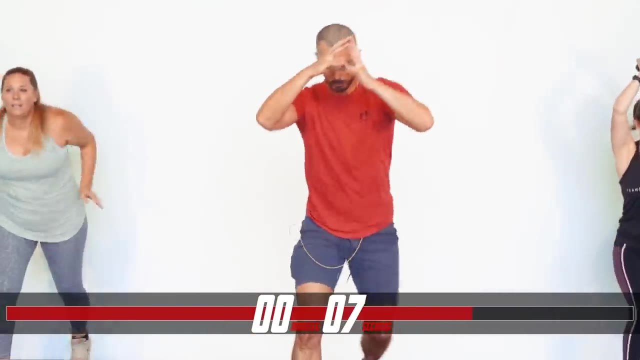 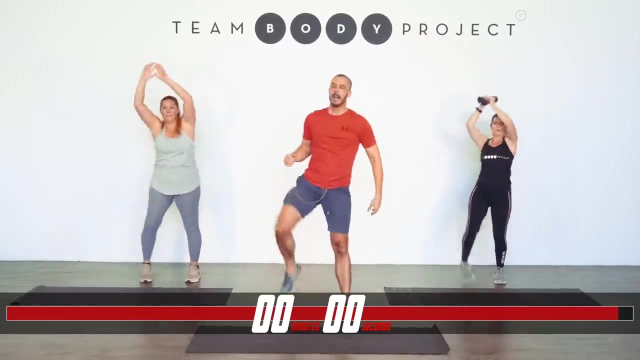 Like you, Do your thing, Your thing. I say it a thousand times: Mute me, Put on some music if you don't want to hear it. I want you to know it. Keep it going, Keep it working. Three, two and one. 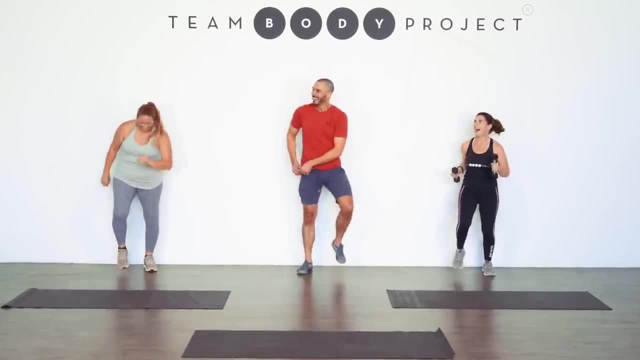 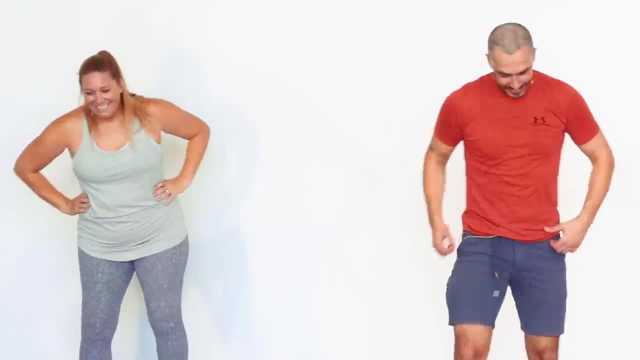 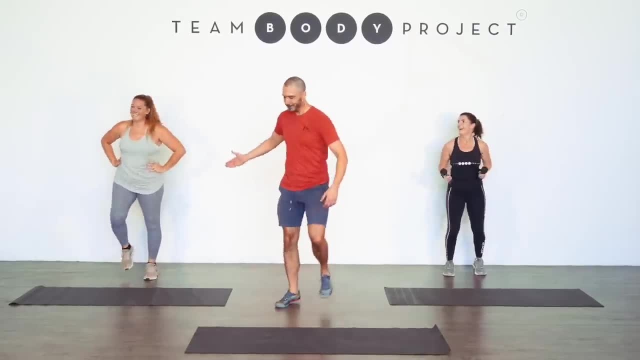 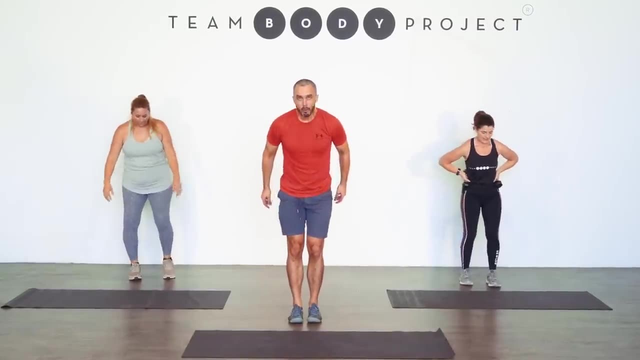 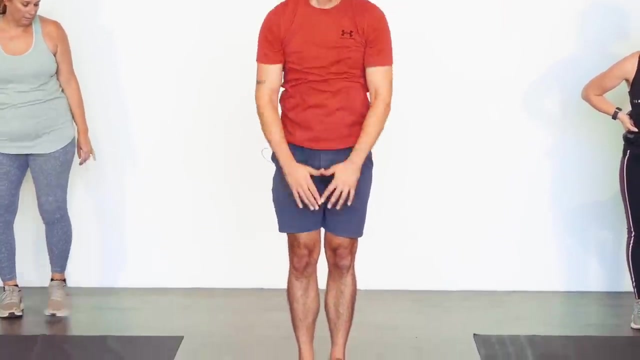 They're like, oh, got more Good. Disappointed, You're hoping that was it. Okay, so let's just get our feet together And what we're going to do is we're going to go on tiptoes and reach high. Now you can just go on one tiptoe at a time or you can do both. 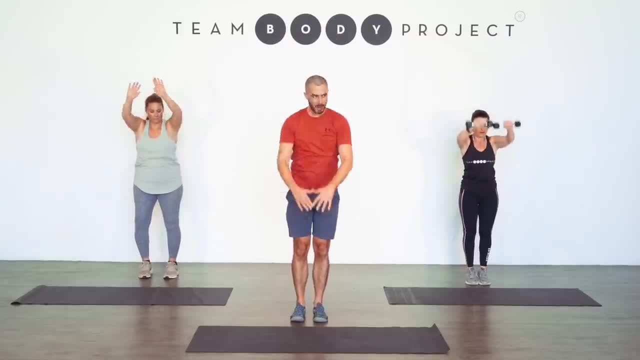 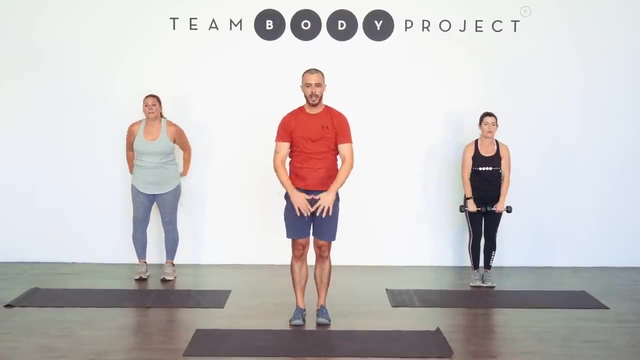 You can count, You can join in. It's okay, There we go. So we're just going to do about 30 seconds of this. So really control the core. This is just releasing the body, Opening up, And if you don't, if you're not able to go on tiptoes because you haven't got the balance, 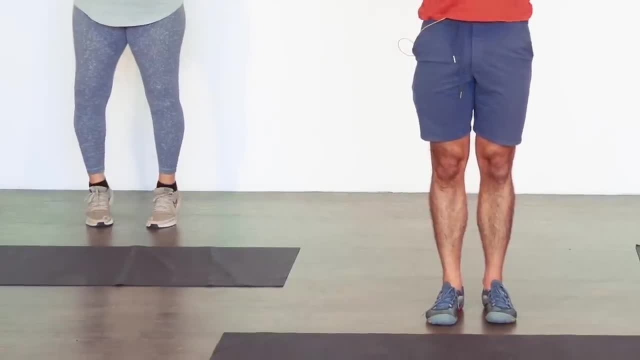 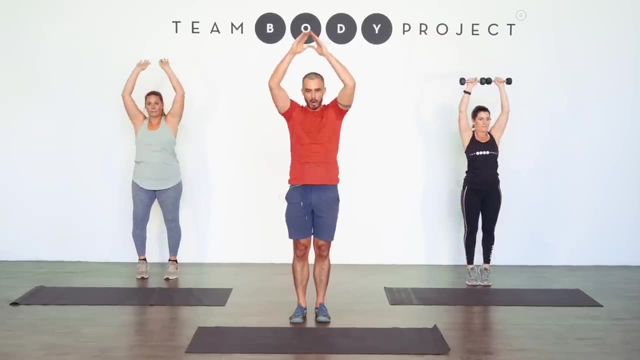 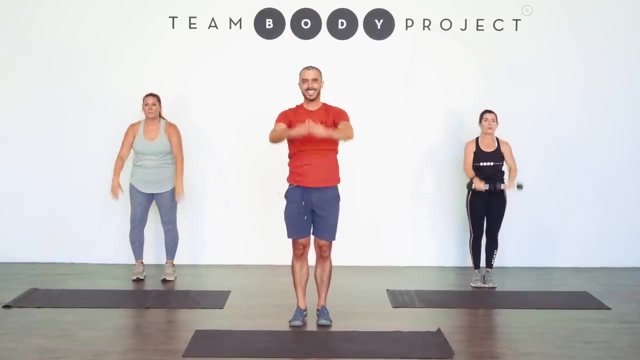 yet. that's normal, That's okay. Stay here, Just opening the body up and breathe, And what I want you to do in these moments is think about where we're going to be for this next five minutes or so, where we are going to take our body to the place that we can. 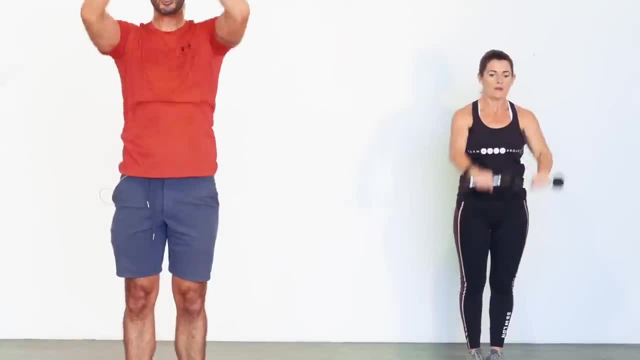 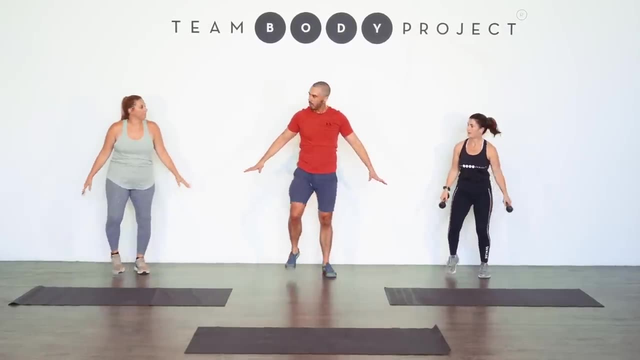 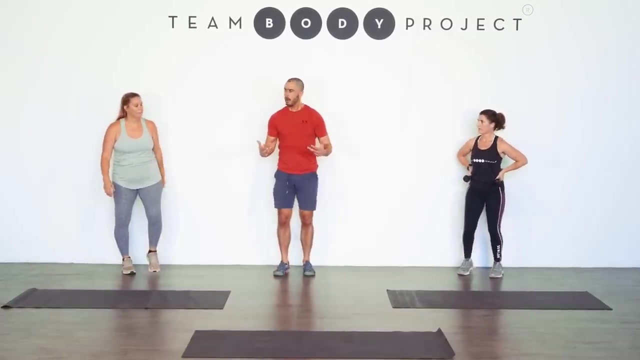 And that will change day to day. Shake it out. So each exercise has got two parts to it. It's got the engage, where we're really going to think about how we're moving, And then 45 seconds we're going to pump it to our best And we can pause whenever we want to. 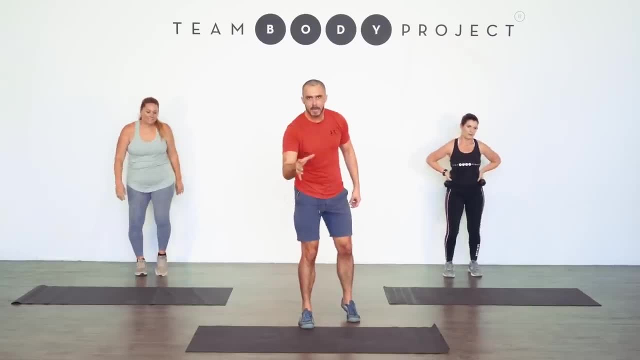 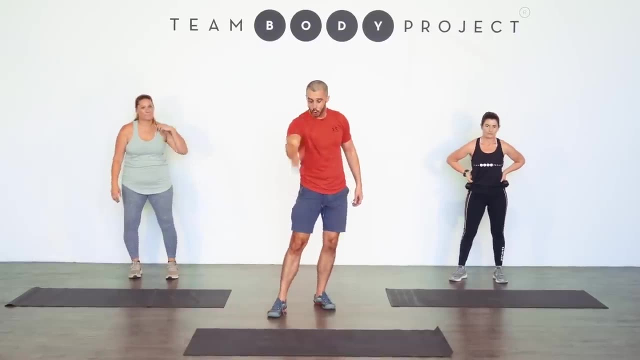 Remember that: No winning and losing, Only taking part. That makes you the winner. So we're going to start with a star jump. I know you've got your own modification for this, And that's good. Three, two, one, So here's the star jump, and with the star jump, 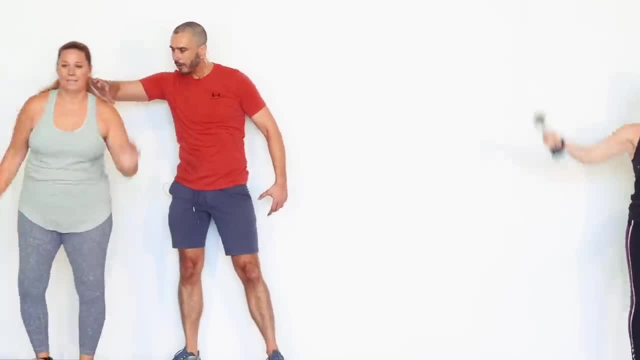 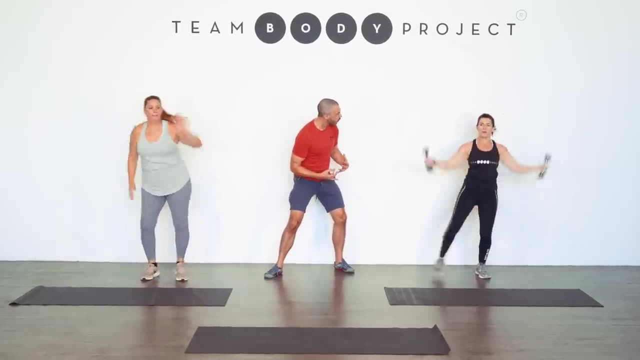 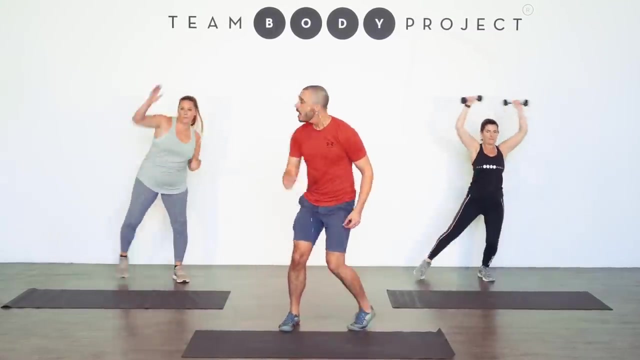 I'm actually going to walk around. We're really feeling it in the side of the body: The shoulders, the side glutes, the side of the legs, the core sucked in tight. Really feel the muscle as it's working, Build a relationship with your body, Feel it, Tune into it And when I say go, 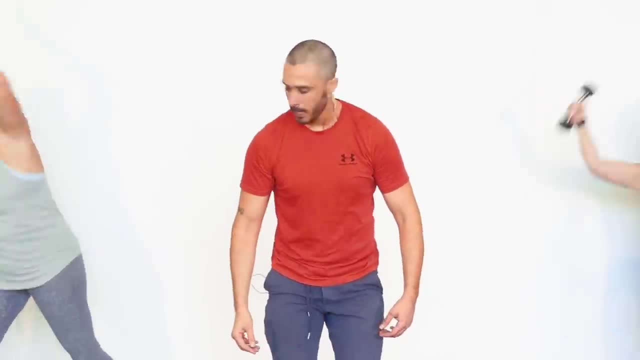 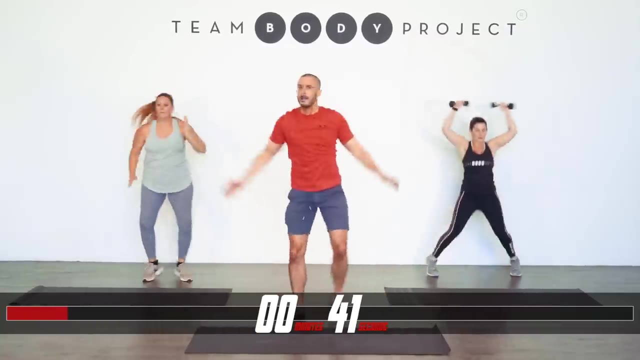 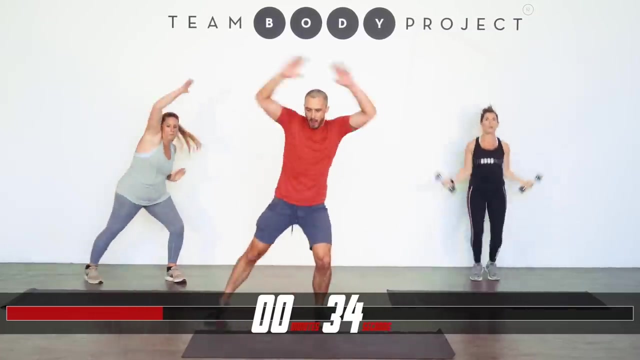 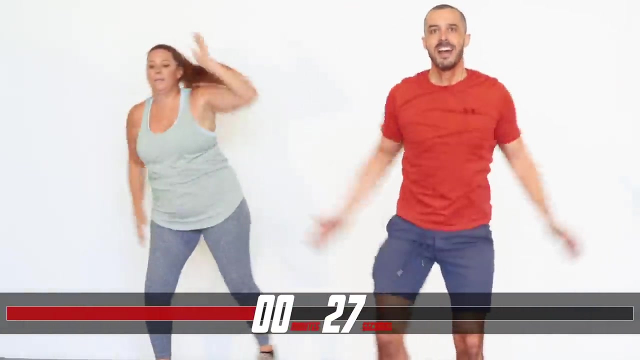 take it where it can go: three, two and one. Here we go: 45 seconds of our best effort, thinking about the muscles. If you stop enjoying it, pause. but if you're enjoying that feeling of testing your body, of using it, of learning how much it's capable of, how incredible it really is. 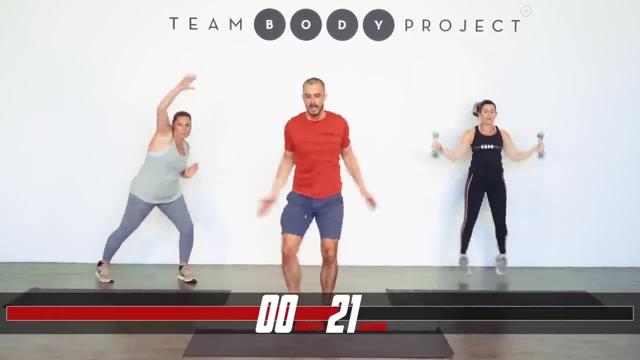 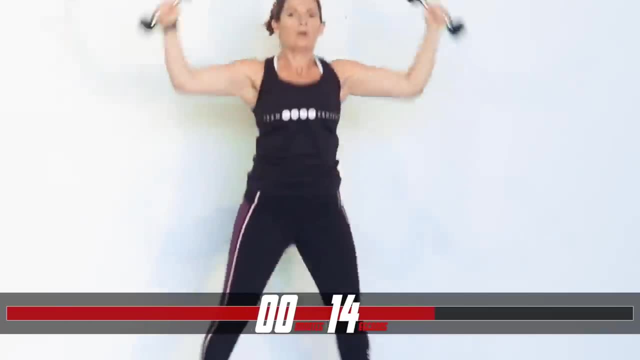 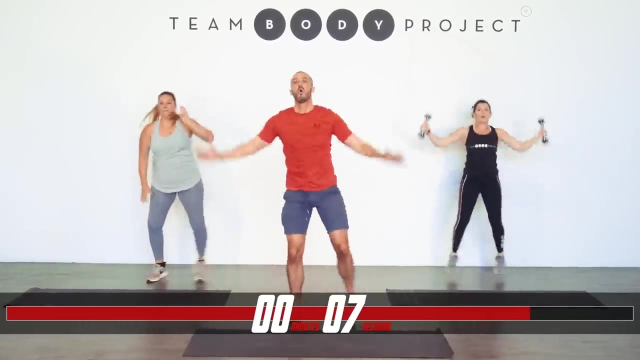 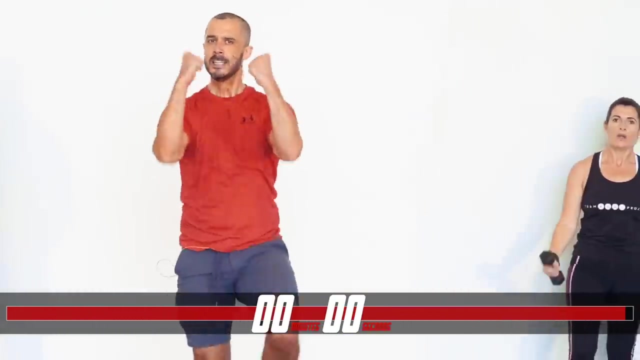 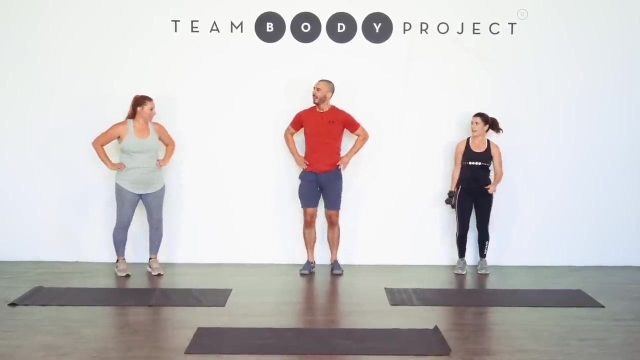 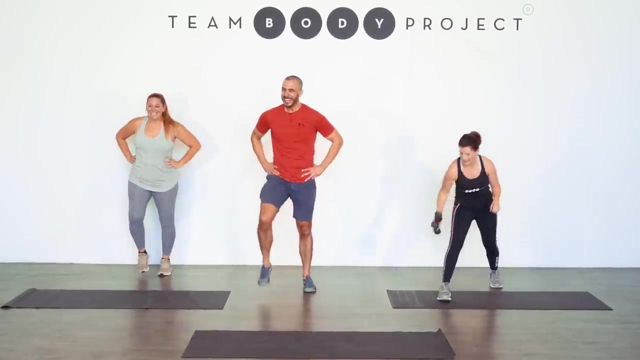 it's 45 seconds. We're almost there. Keep pushing, Here we go. This is mental. now It's no longer physical. What can you bring? Three, two and one Deep breaths. Feel good, Feel good, That smile authentic. 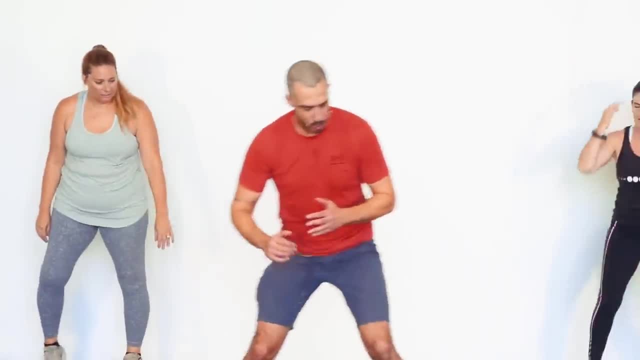 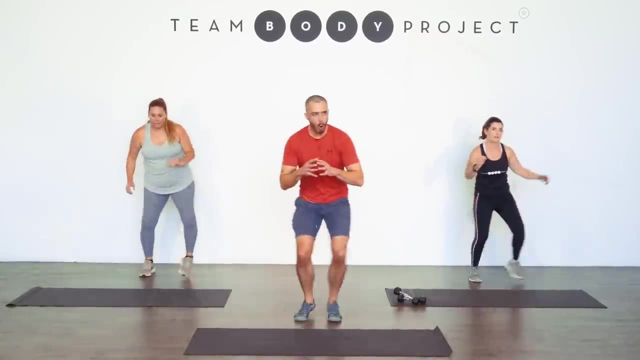 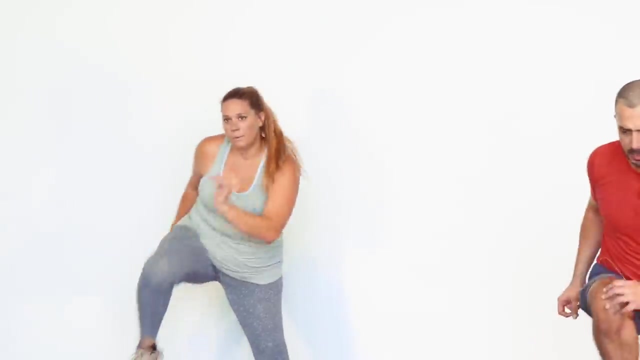 Okay, football drills next. We're just going to step it across. Feel it Low, sit, Feel the glutes, Feel the quads, Feel the core, stabilizing your body, Tune in Every movement. Yes, Feels good, doesn't it? Look at what you can do, Look at what we can do. 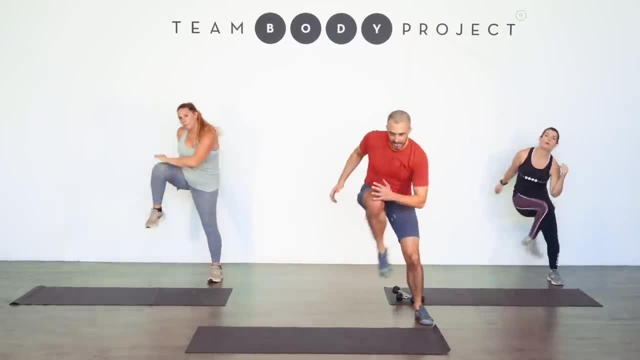 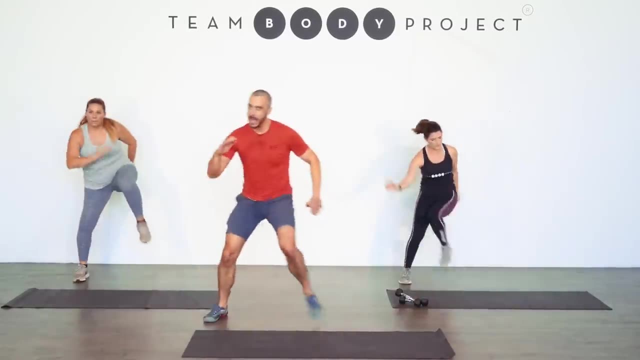 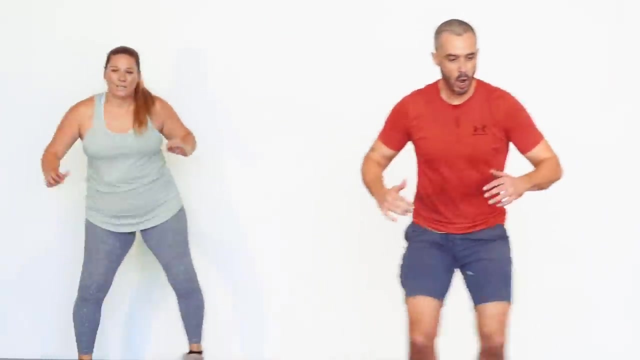 This body that gives us everything: Protect, Nurture, Grow, Live, Love. You name it. it all happens with this body. Now let's see where we can take it. Let's give it some payback, Let's show it what it deserves. Three, two, one. How can you go now? 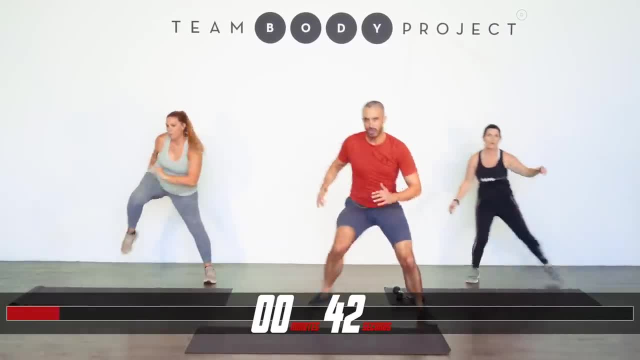 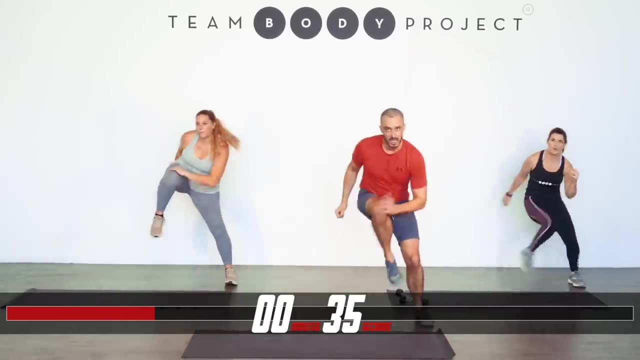 How can you go Your best, Your best, Tune in, Tune in. This is a challenge. Your body thrives off of it. If you need to pause, you're still winning. Don't worry, You come back in and you give your best. 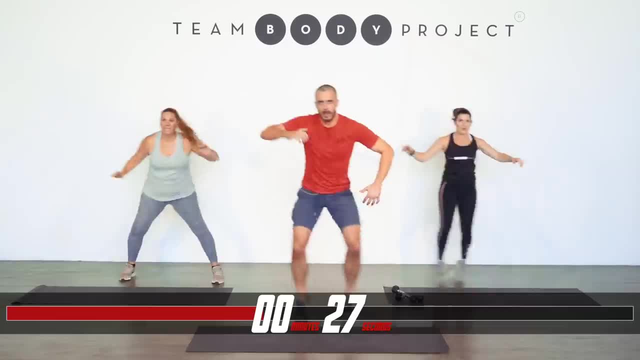 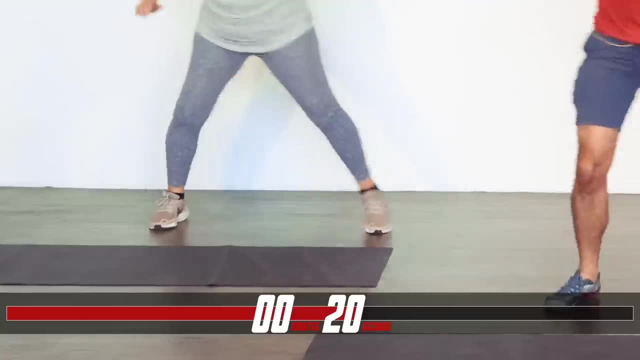 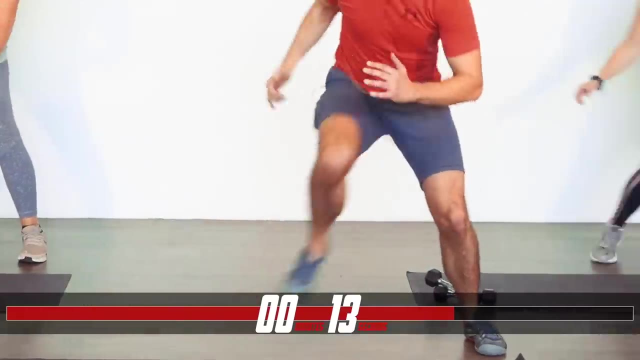 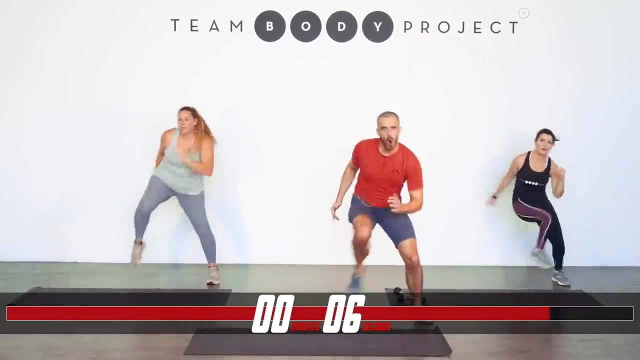 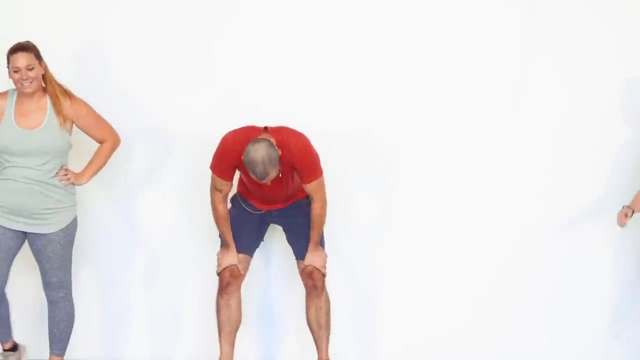 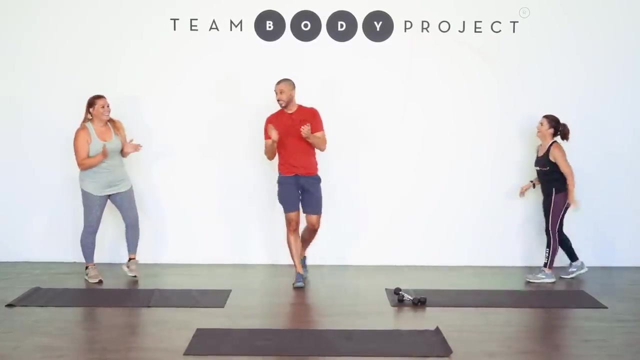 whenever you're ready, Come on, Focus, focus, desire, drive, determination, Determination, fight, five, four, three, two and one, Yeah, yeah, yes, You see where it can go right, We're not done. 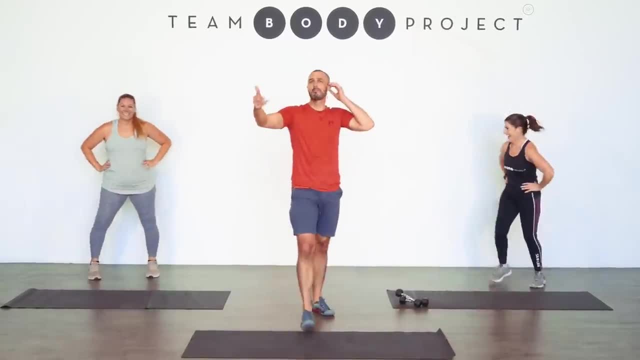 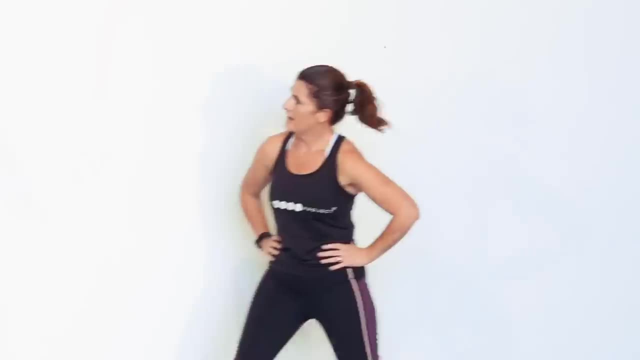 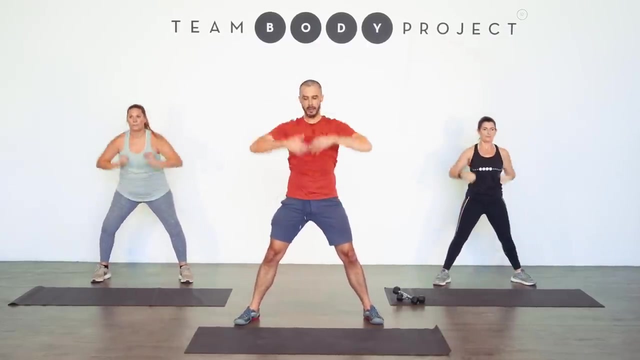 Hey, where's the high fives? I see the body, Body project, high five and it's not come. Touch and raise next Again, we don't need to touch the deck. Three, two, one Shoulders proud, sit down and lift high. 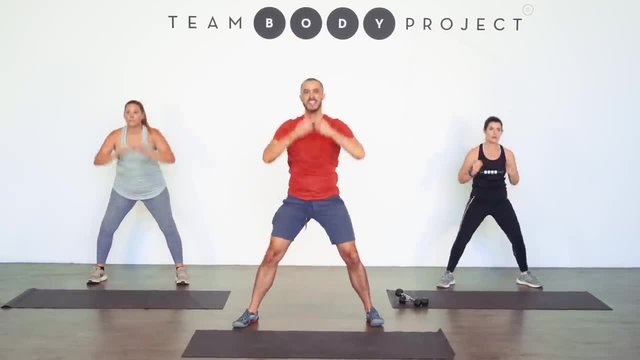 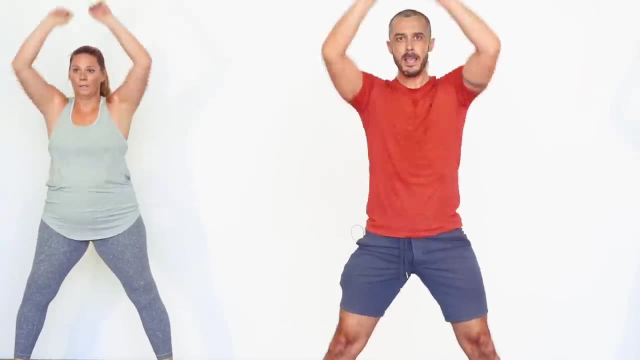 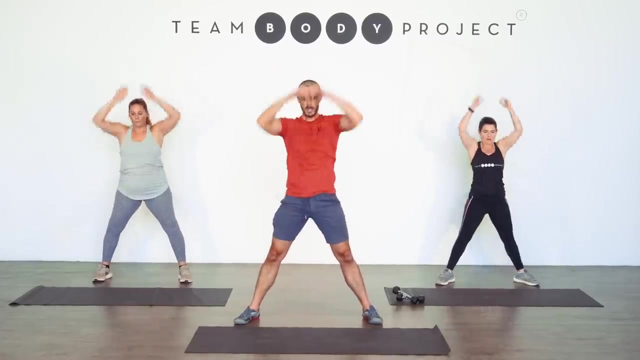 Reach high, as high as you can Suck the energy in 45 seconds of this is the real deal. Be ready, be prepared, be focused. Working through now Three, two, one, Your personal best, That core, strong mean it. 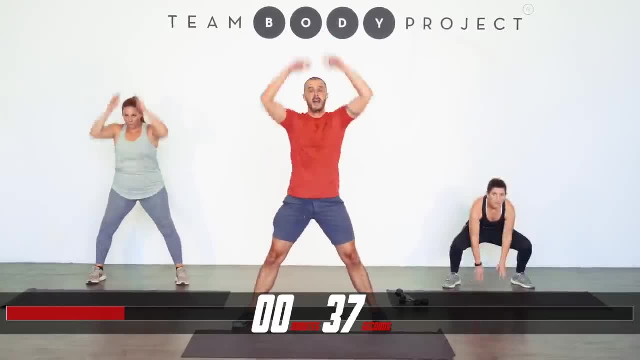 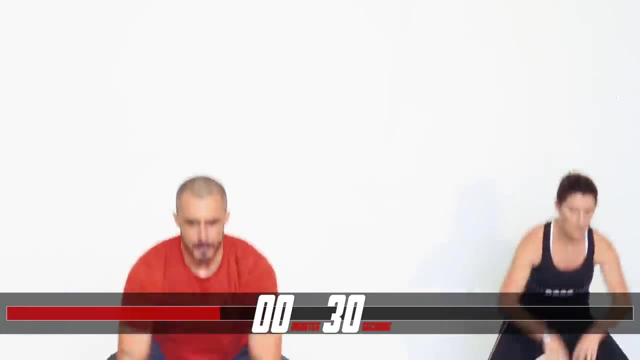 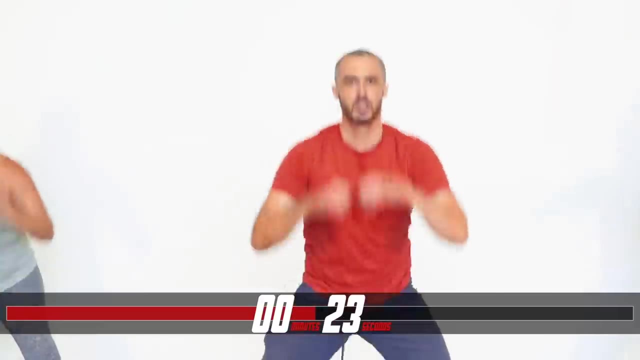 Feel how good your body is. It's going, it's working. You're on fire. Think you did, Come on. come on, Suck the abs in tight, Working through. We're almost there. Dig, dig, Find it. 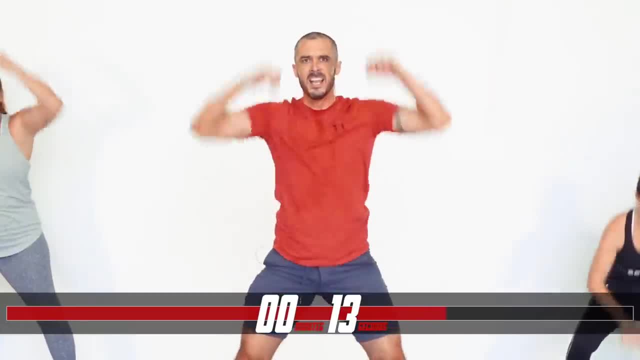 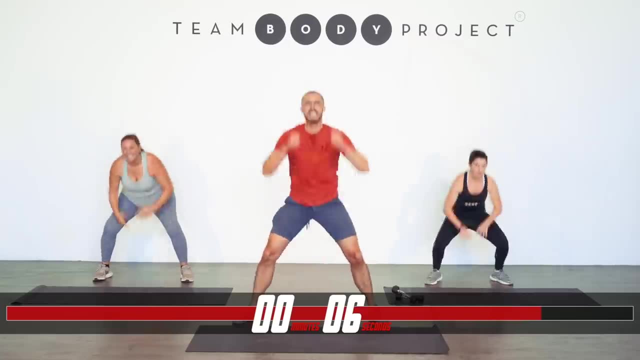 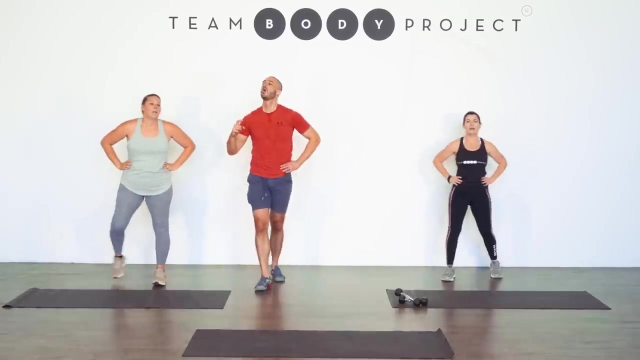 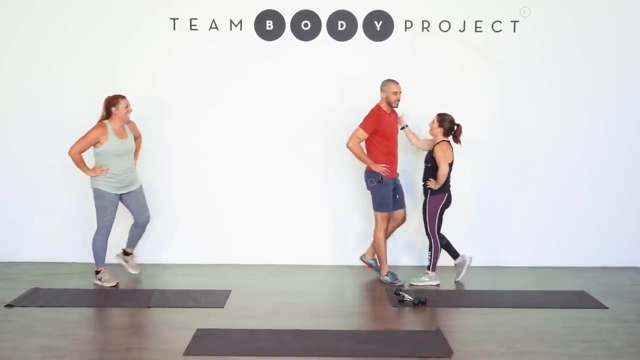 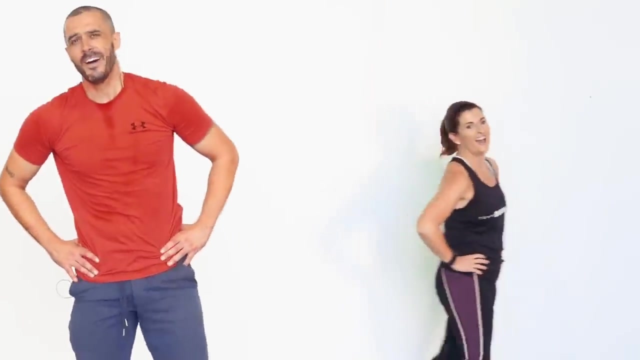 Find it from somewhere. I know it's there. This is what it feels like to win. Ah, Come on. Ah, Three, two, one. Oh, You're still enjoying it, Are you still enjoying it? Just, I said to Kristen: don't worry, it'll be fine, it won't hurt, but it feels good, it feels. 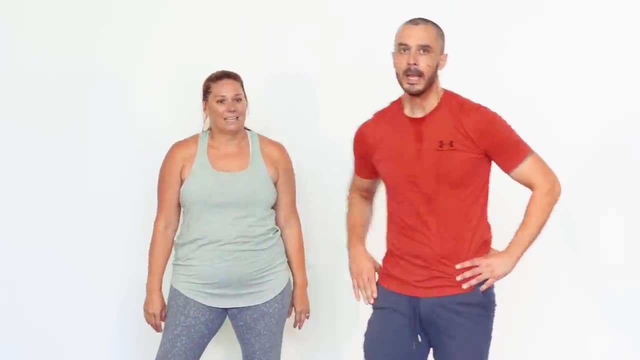 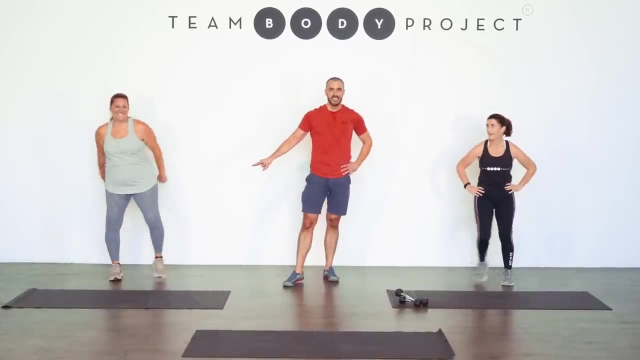 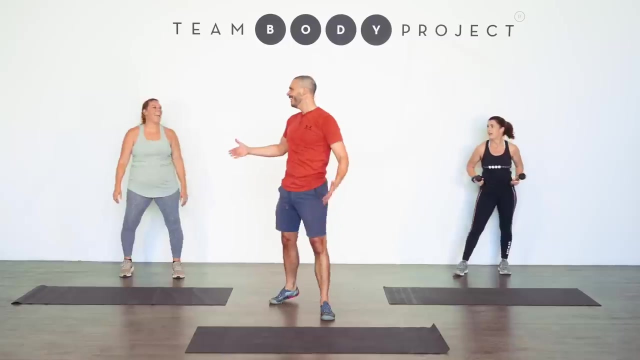 good, the pain doesn't it? you're in there, you're with it. okay, let's finish with the punches and this is going to bring the high five. I promise at the end we'll do a central high five. we'll pre-prepare it so it looks at least a little bit Hollywood. we're not. 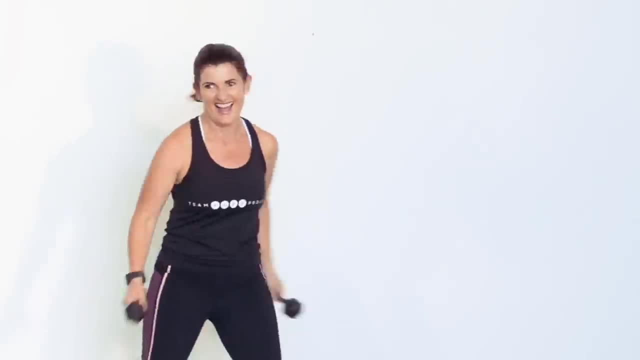 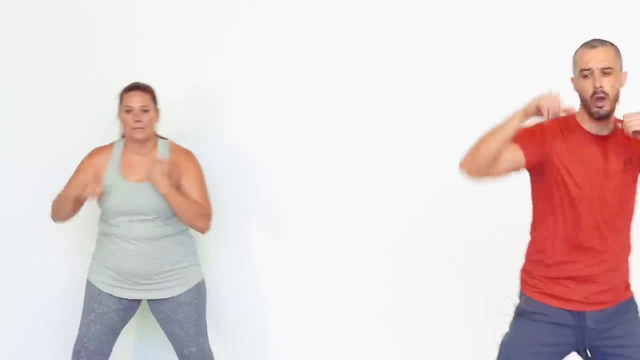 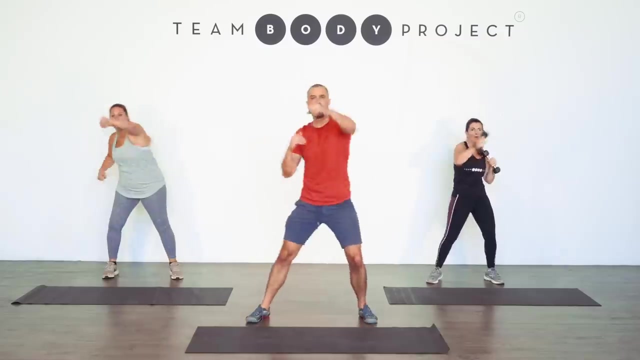 good at that. a body project. but okay, three, two, one, so full extension on the punches. just feel how long your arm can go, tune into it, feel it. look how the hand is extending all the way out. every part of our bodies are moving. your steps, there is good get. 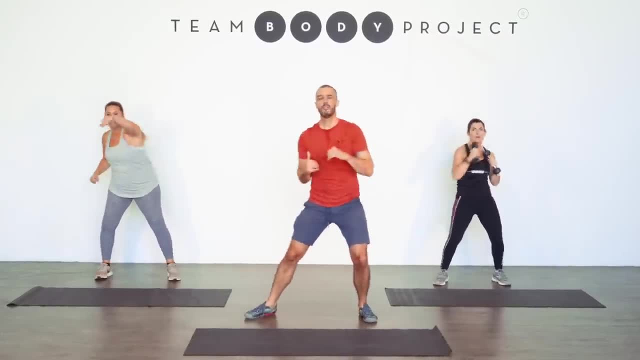 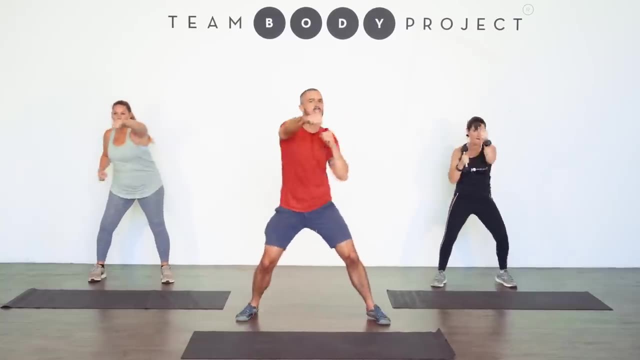 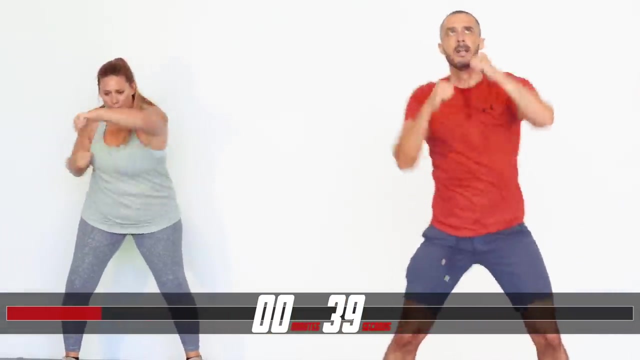 that core strong. everything's working. now let's pump this. 45 second finale. this is where we get the warrior badge. three, two, one. Here we go. here we go. as much as you've got, do not leave it here. do leave it here. 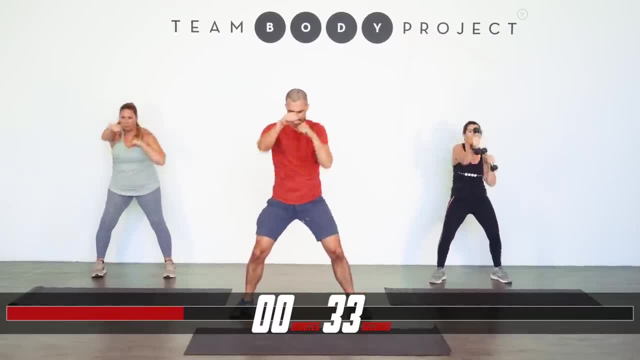 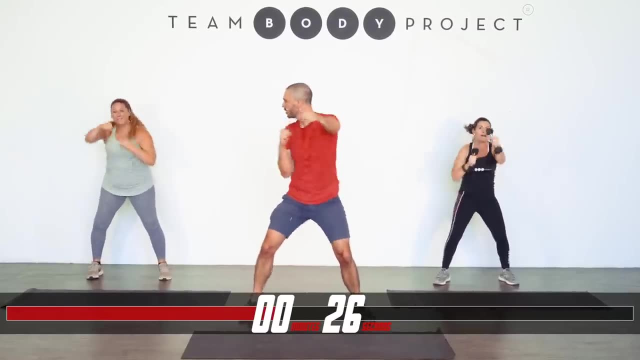 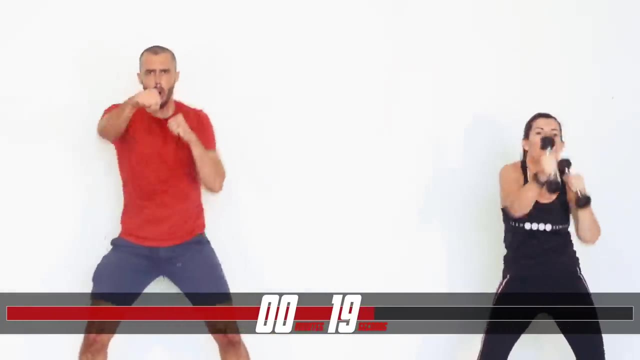 don't take it with you. that's the right way round. come on, come on now, fire up, fire up, go to that finish line. go to the finish line, Kristen, go all the way there. come on, come on, Tash all the way to the finish. everything this is what your body can do. 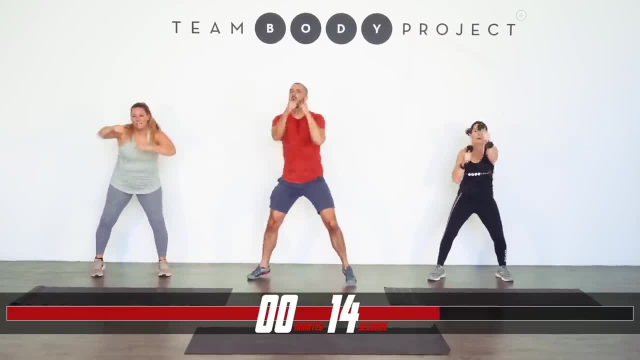 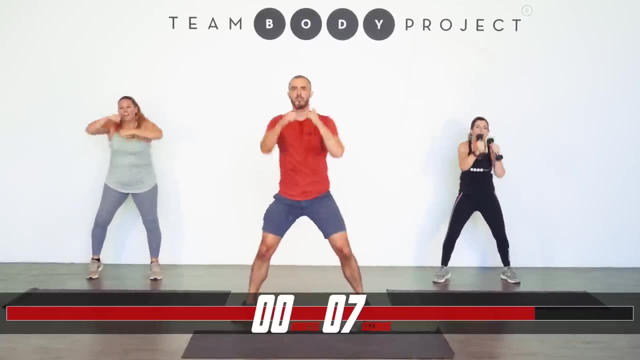 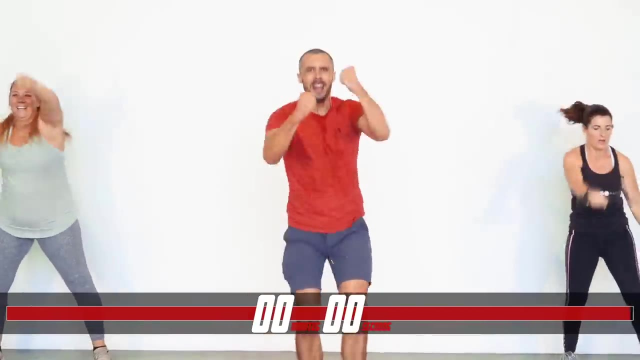 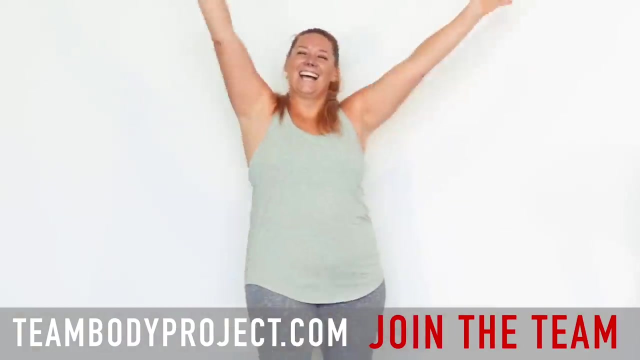 show us, Show yourself, what you've got. it's inside, it can't be quantified, it can't be measured. it comes from the spirit, it's heart. show us three, two, one Central. oh oh, oh dear. I'm so pleased that someone's finally here. I'm so pleased that. 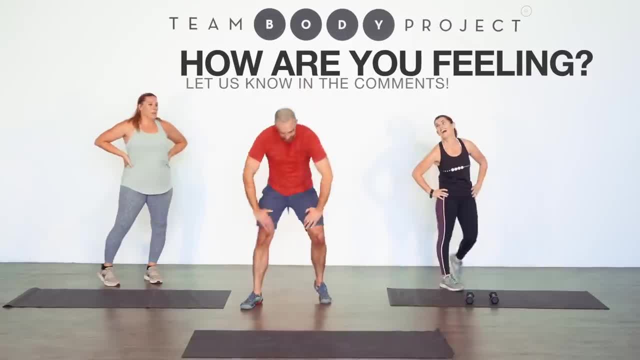 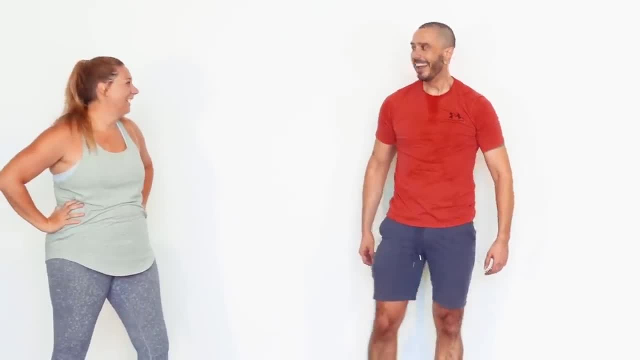 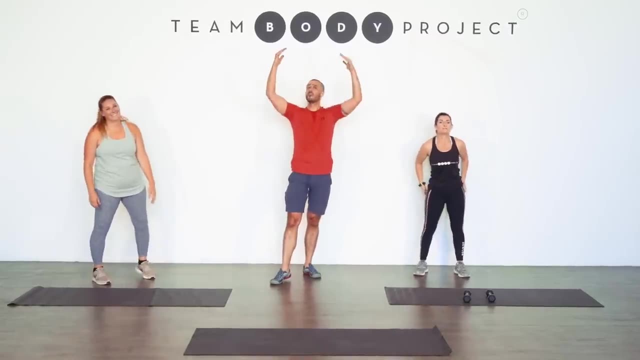 someone's finally come along who does the same bend over as me. How good was that. Yeah, that was a pretty special session today. your energy- both of you and I know yours- was off of the charts you really took. it's the first time you worked out with us you. 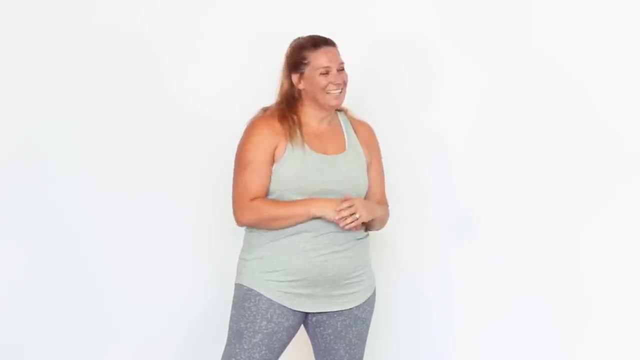 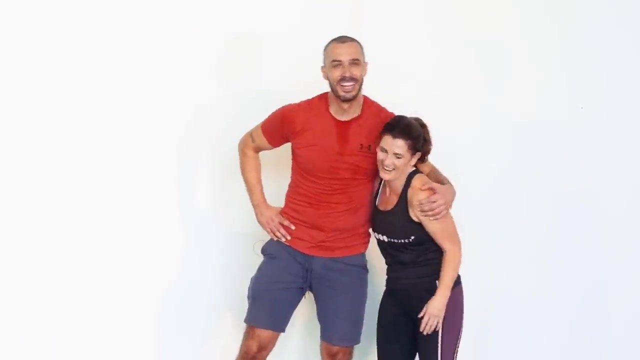 took every word and you took it with you. it was amazing. it was so good. I'm so proud of you. honestly, that was amazing, And you, of course. Of course as well, Tash, but I've said that to you a hundred times, haven't I? 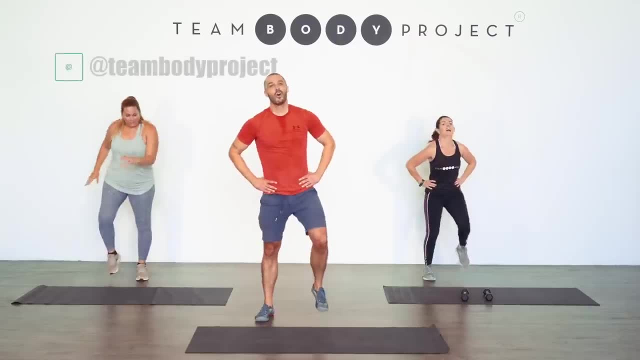 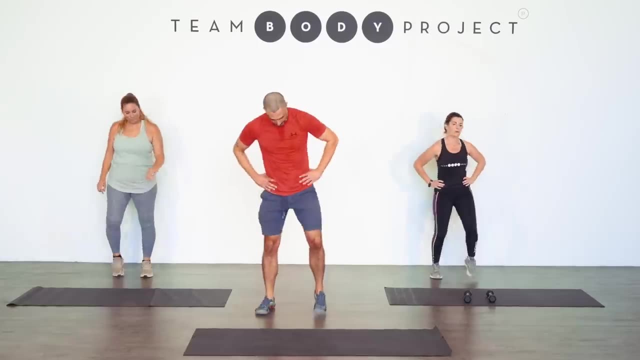 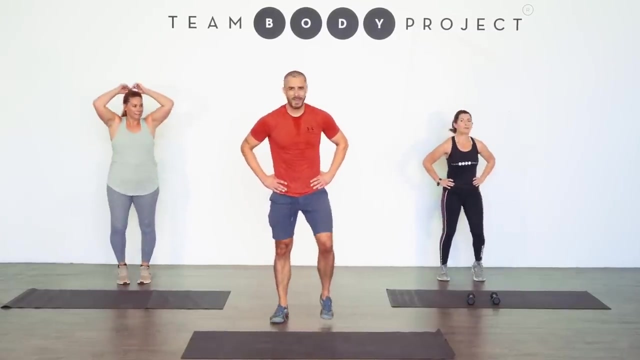 Okay, good, All right, let's get marching. we've still got a cool down breathe in there. The words I used throughout that workout, and I know I used them again and I repeated them a thousand times, and I'm fine with that. you've got a mute button, I don't mind, but 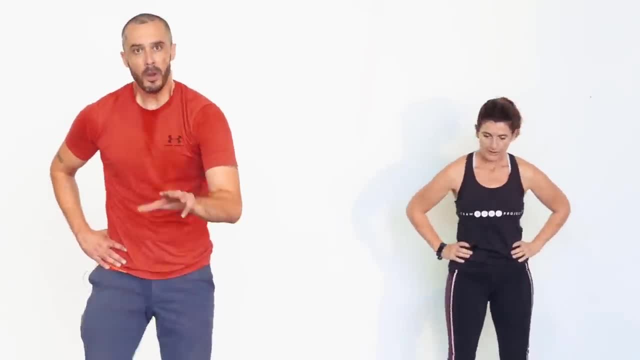 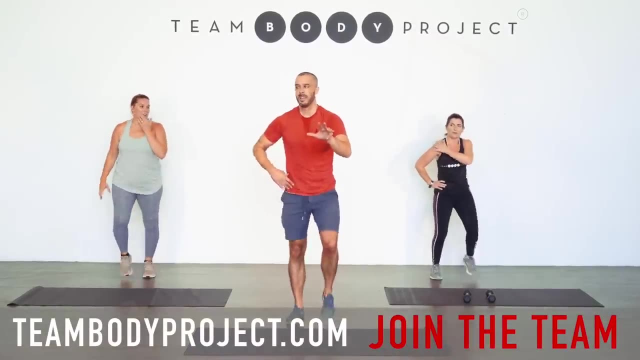 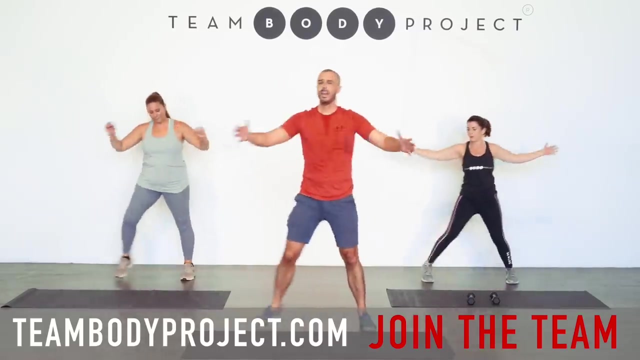 the reason I do that is because it's the truth. Our bodies are fantastic and we've got to remember that Exercise isn't punishment, it's joy, it's moving- this wonderful thing that we've got that allows us to do everything in life, and this time: 30 minutes a day, 20 minutes a 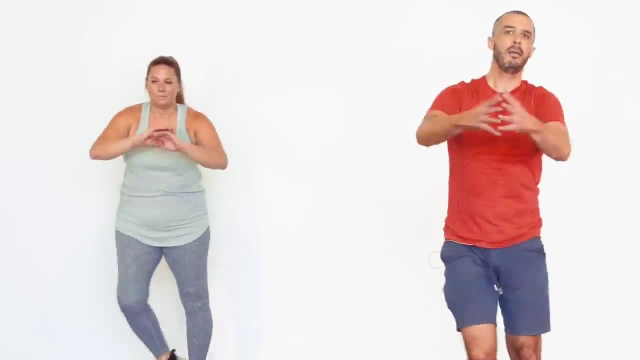 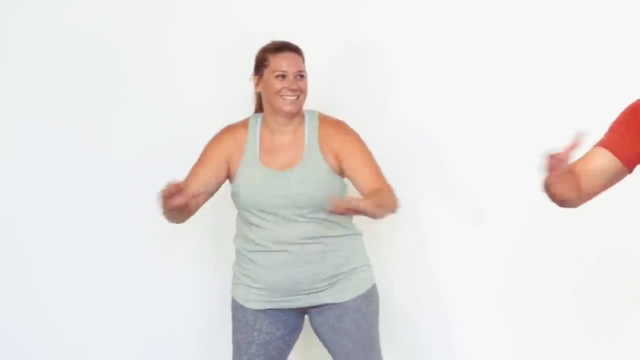 day, 20 minutes, three times a week. it's a time to embrace it and say, wow, this body's pretty special and I'm proud of it. It's the big message I want you to take home, and well done.